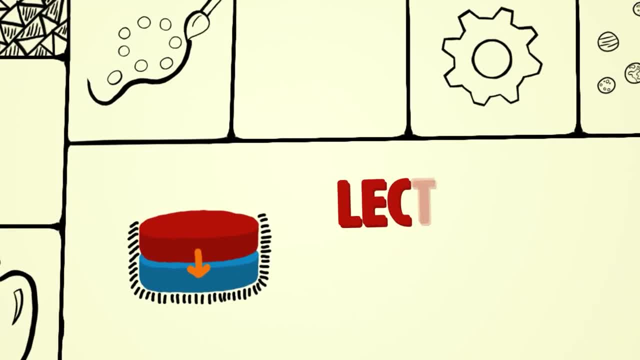 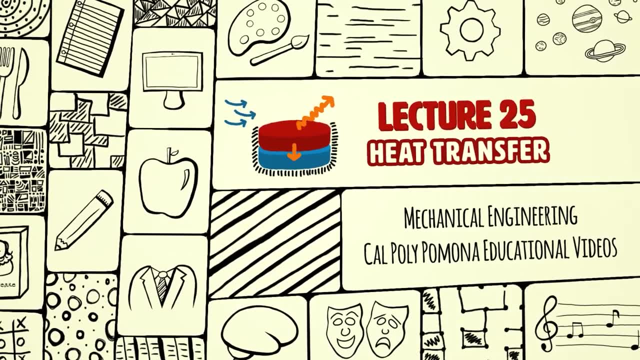 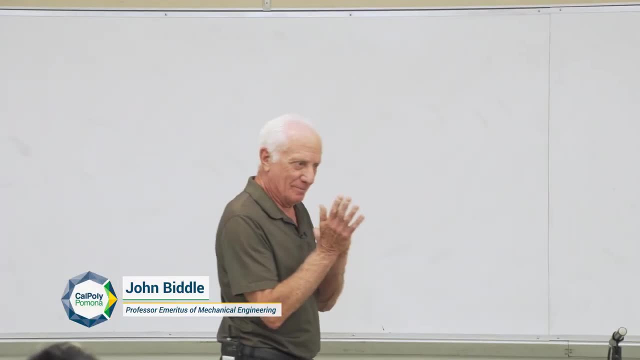 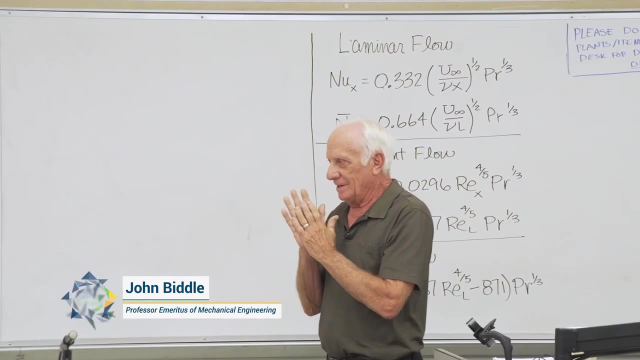 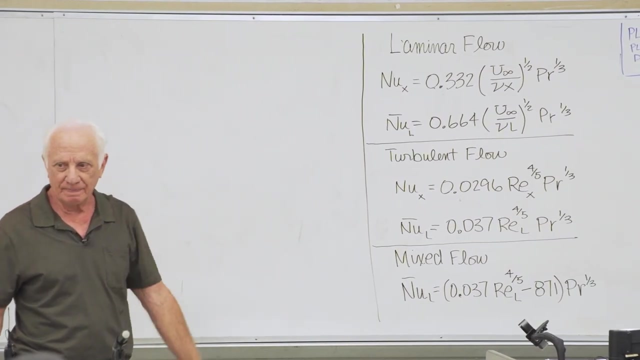 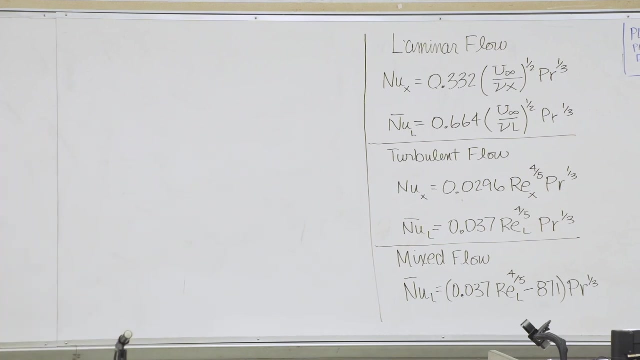 We are in chapter 7, the first part of chapter 7, looking at flow over a flat plate. We covered many different possible flows, from laminar to turbulent to mixed flow, So we're going to use those equations now in an example problem. So here's our example problem. The fluid is water. 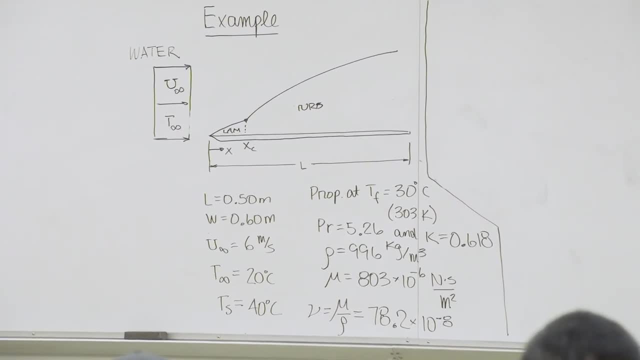 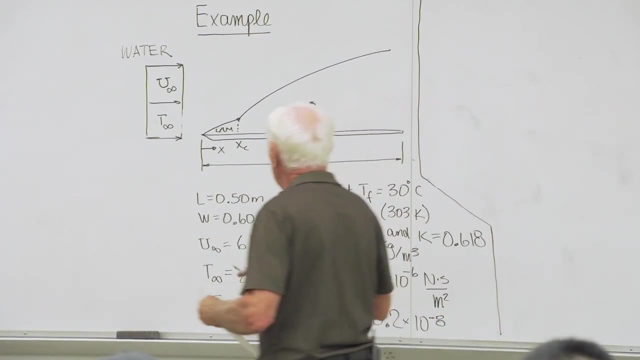 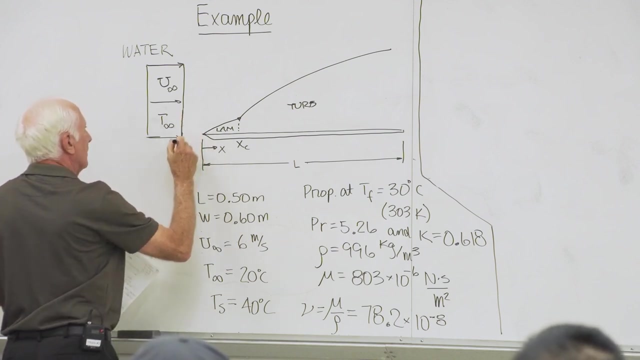 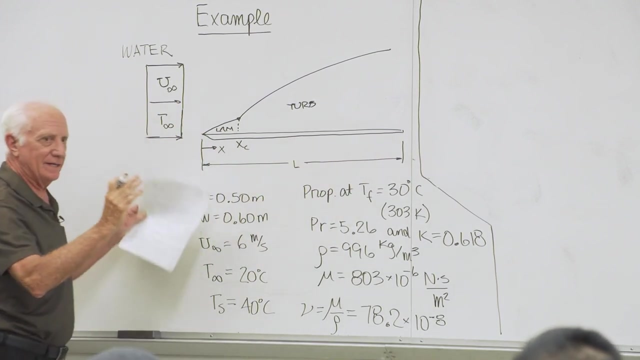 Let me get a pen here. The fluid is water and it has a free stream velocity- u- infinity- And a free stream temperature t- infinity. Here's what we're given. We're given the plate length 50 centimeters 0.5 meters. The plate width into the board 60 centimeters, 0.6 meters. 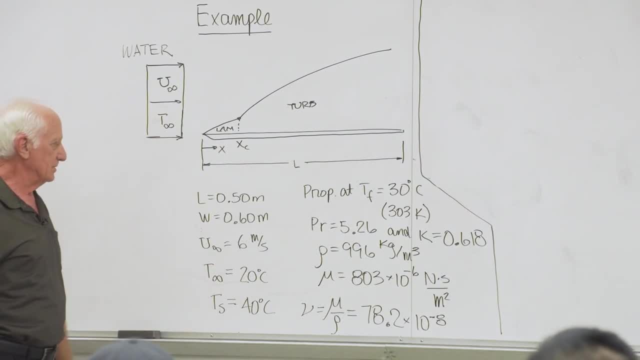 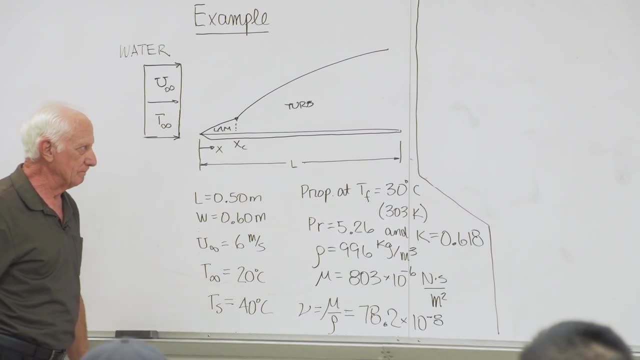 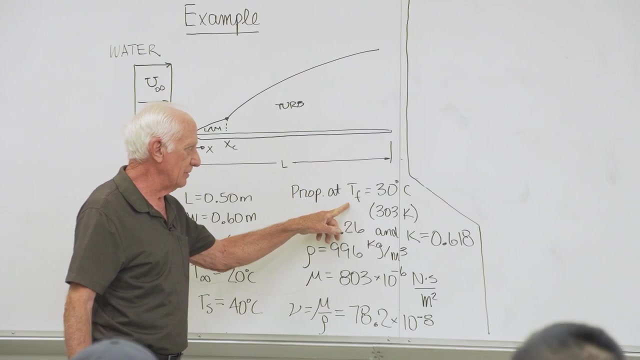 Free stream velocity: 6 meters per second. Free stream temperature: 20 degrees C. Surface temperature of the plate: 40 degrees C. We evaluate the properties at the film temperature, the average of the surface and the free stream, which is 30 degrees 40. 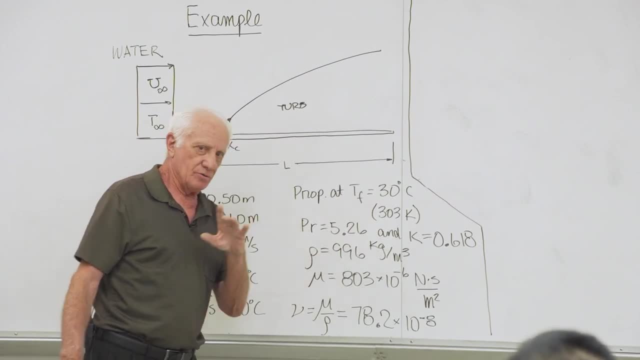 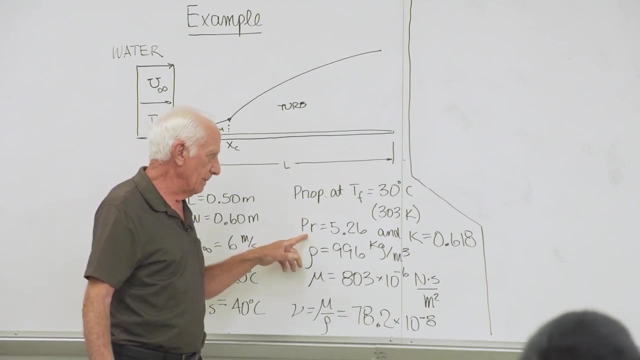 plus 20 divided by 2, or 303 K. We go to the back of the book, to the appendices. We find the properties at 303 K for water, Prandtl number, thermal conductivity density, average temperature and free stream velocity. So we're going to look at the properties of the. 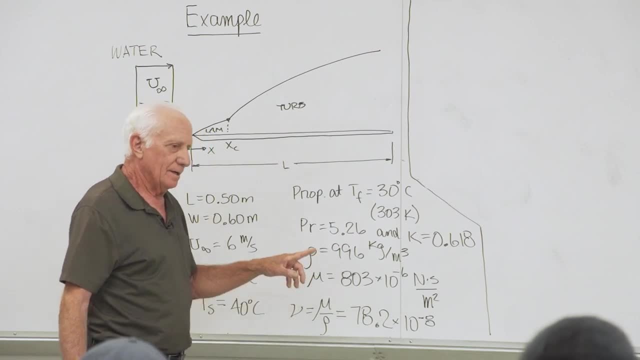 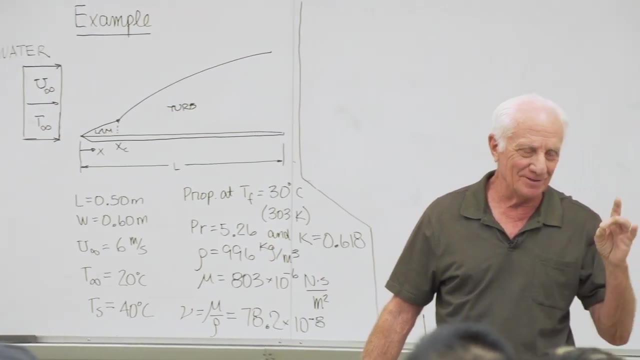 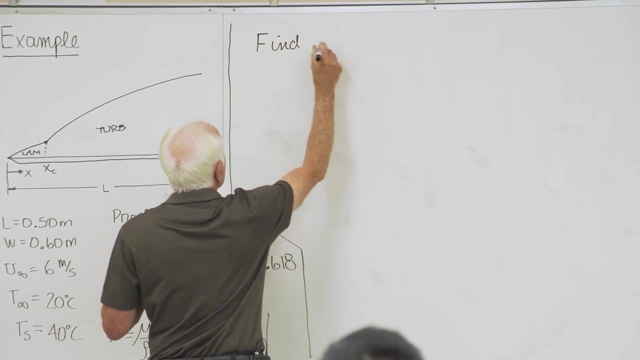 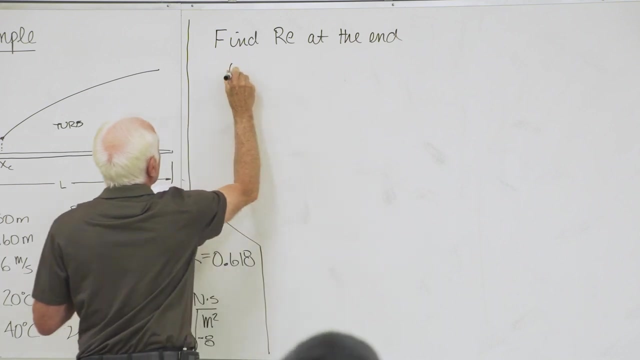 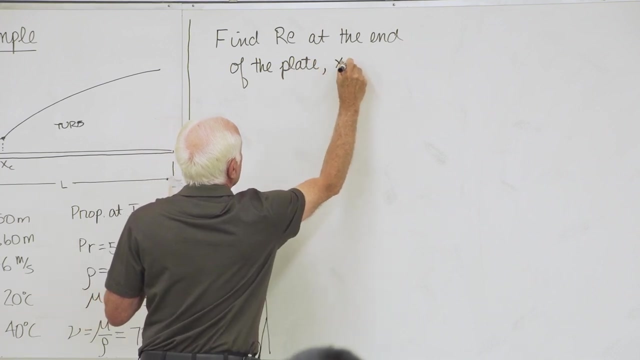 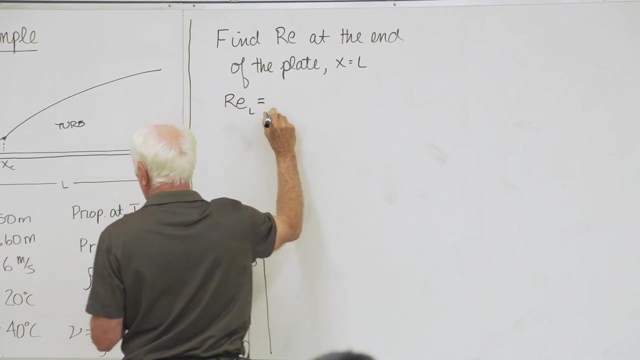 absolute viscosity. Now, the first step in a problem like this is almost always to get the Reynolds number at the end of the plate. So step number one: find the Reynolds number at the end of the plate. X equals L, So R Reynolds number at L is equal to the Au infinity. 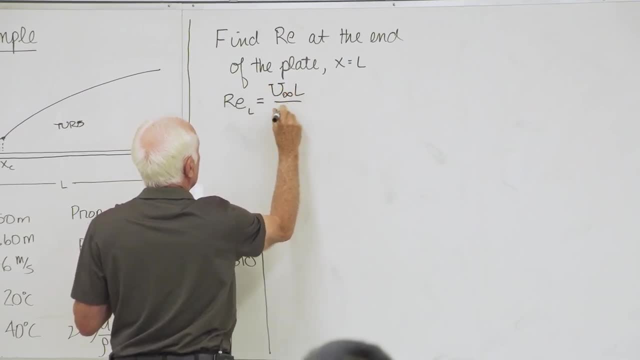 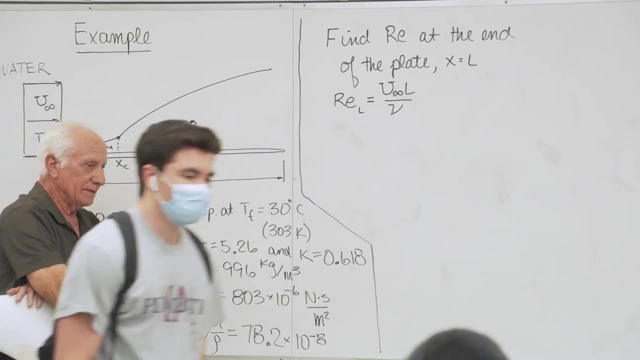 L over new. Now the back of the book and the appendices. you won't find the kinematic viscosity- new, So you can calculate it from fluid mechanics. New equals zero. Second step: there that's finiteugar. So this is independent. and now that's V. And now that stated, there's some expression. that the front is here. its an non- Face. What you do is you actually do right. You either figure it out that there x is constant, or but it's not a constant, and values you can multiply or plus or minus, and you have to do it whatever effects they have. So, as you, 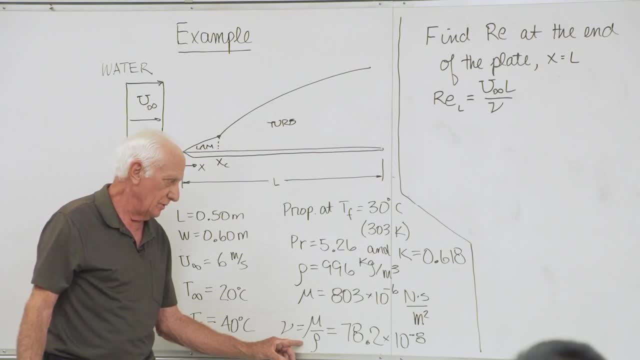 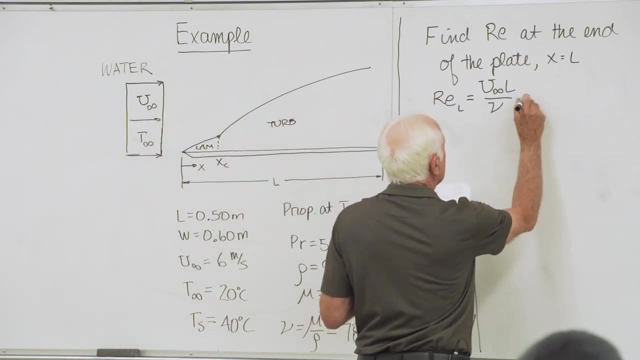 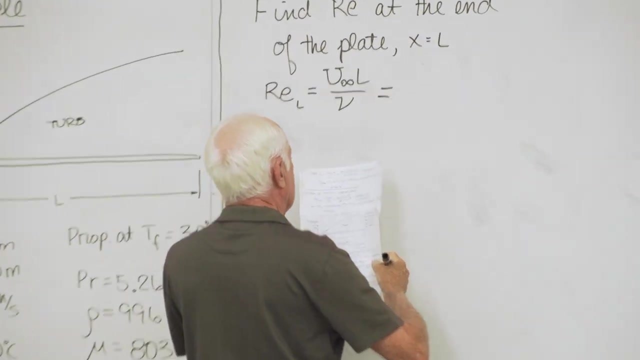 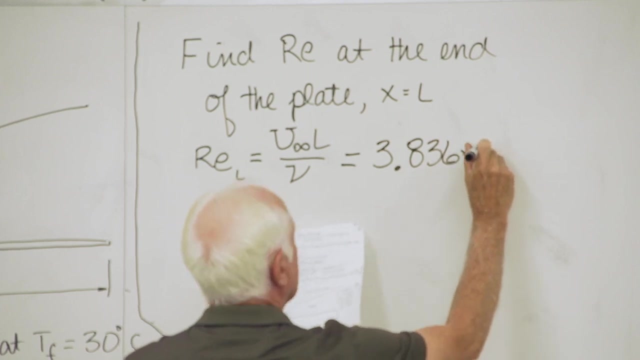 equal mu divided by row. When you do that, you get this guy, So now you've got everything you need here. The Reynolds number at the end of the plate comes out to be 3.8636 times 10 to the sixth. 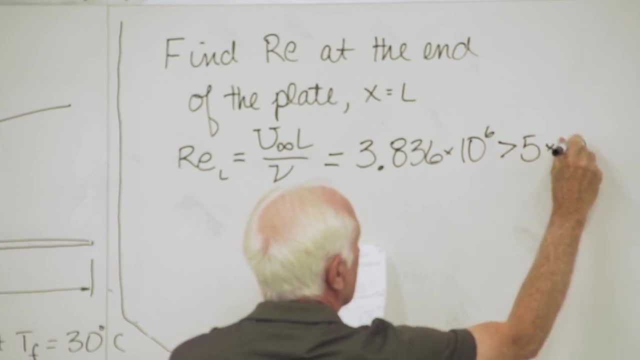 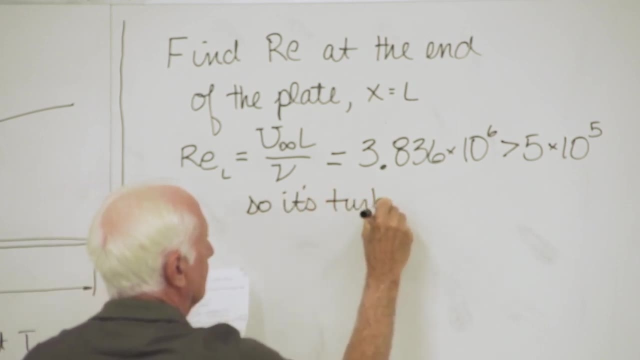 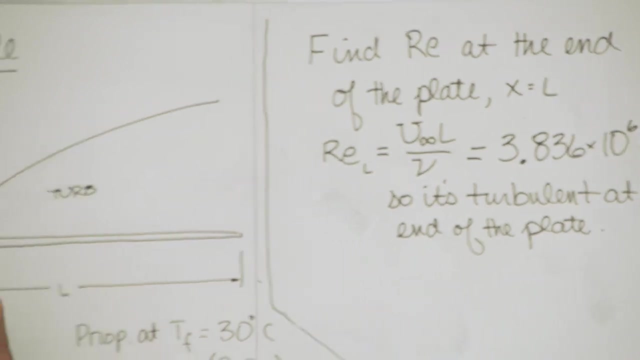 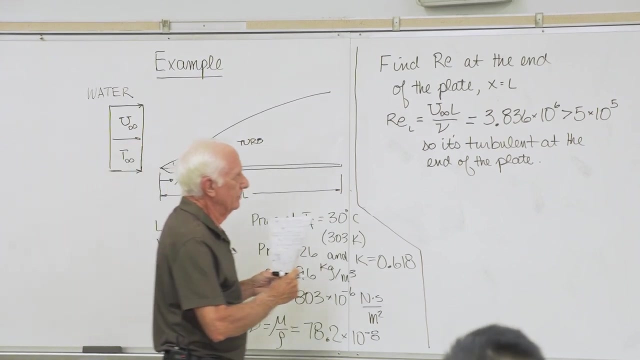 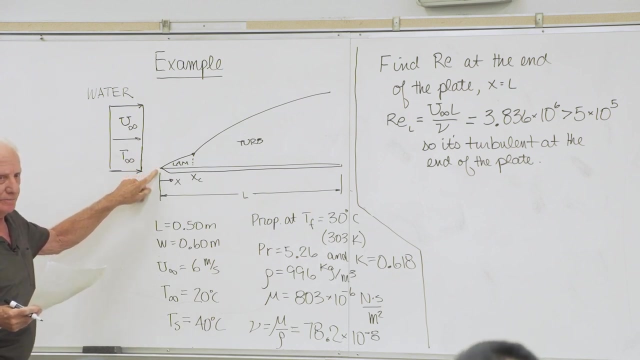 greater than five times 10 to the fifth. so it's turbulent at the end of the plate. Well, that tells us right away that it's mixed flow, because the flow starts out laminar from the leading edge. x equals zero. How do I know that? We know the rule I said. 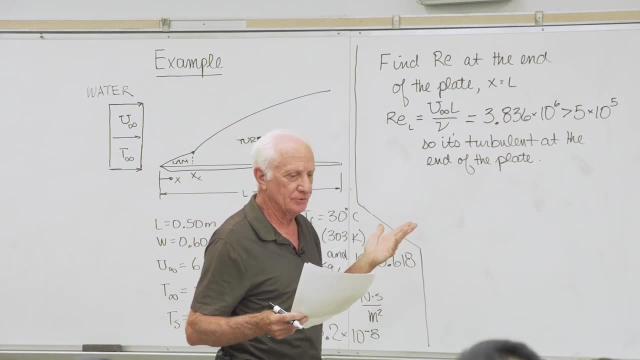 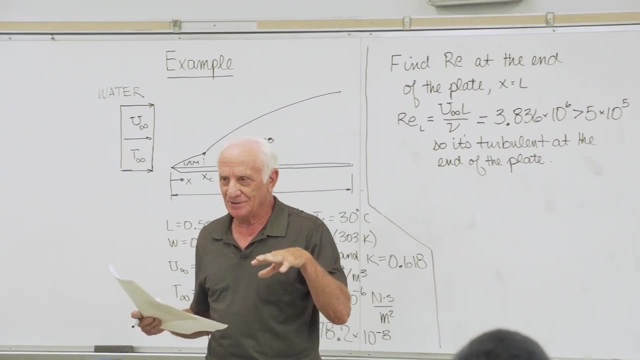 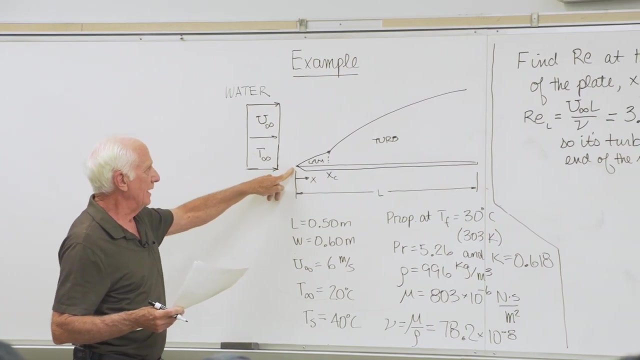 In the textbook. homework problems are in-class examples or a quiz or exam, Unless somebody says the flow starts out turbulent from the leading edge. If they don't say that, assume the flow starts out laminar and then if it's turbulent at the end of the plate. 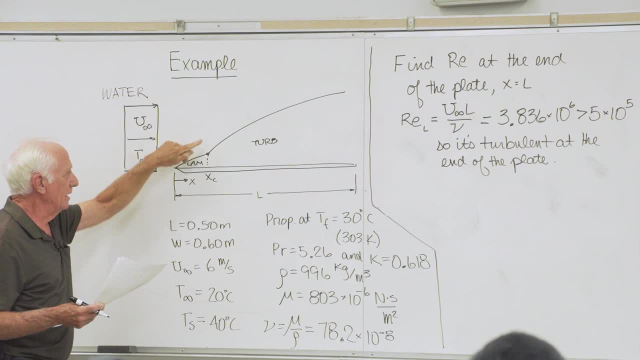 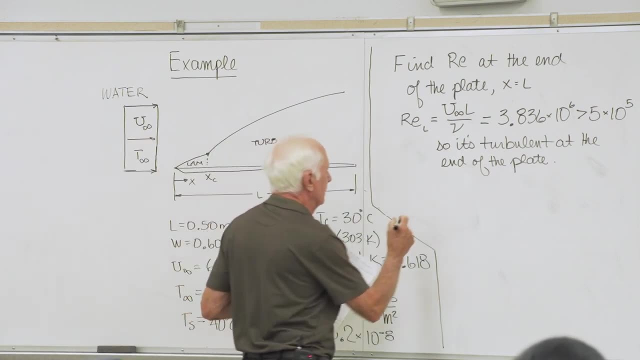 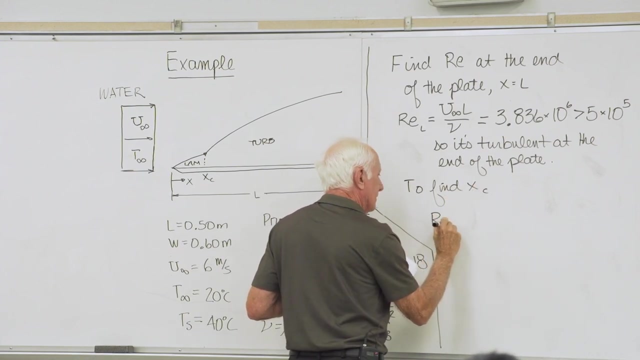 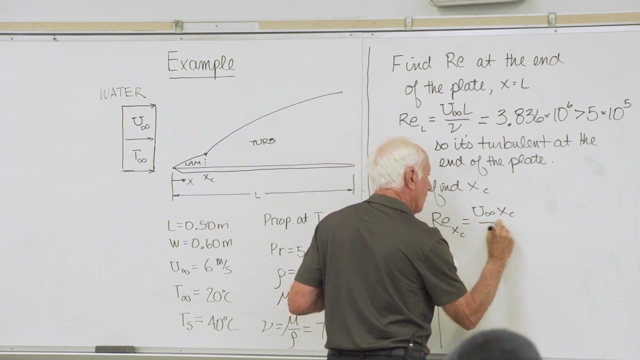 it has to transition from laminar to turbulent flow Where At the critical x value x sub c. So now we know this, Now we find x sub c. So to find x sub c, Reynolds, number xc, u, infinity xc over nu. 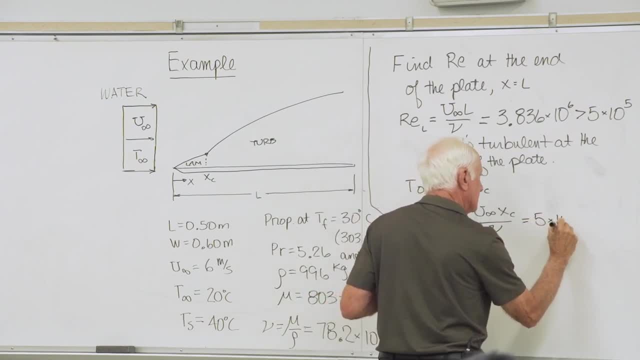 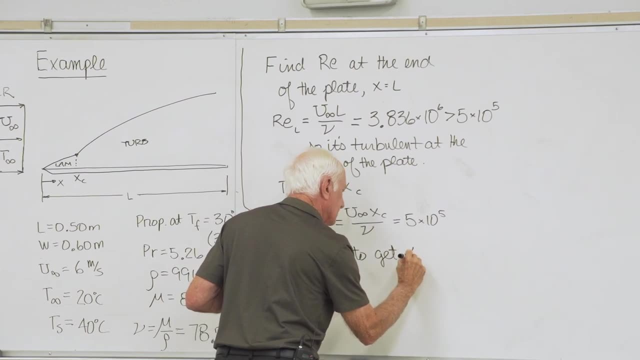 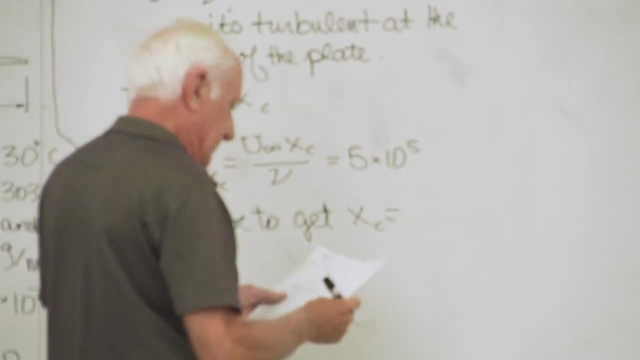 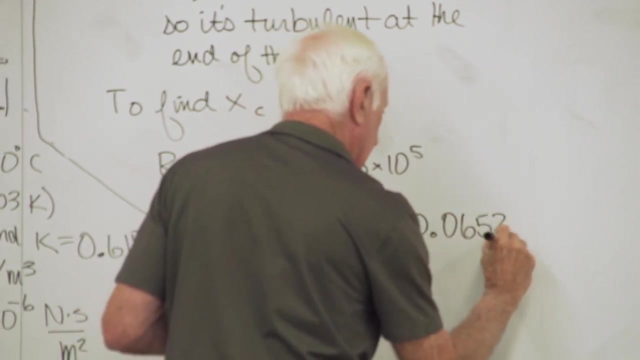 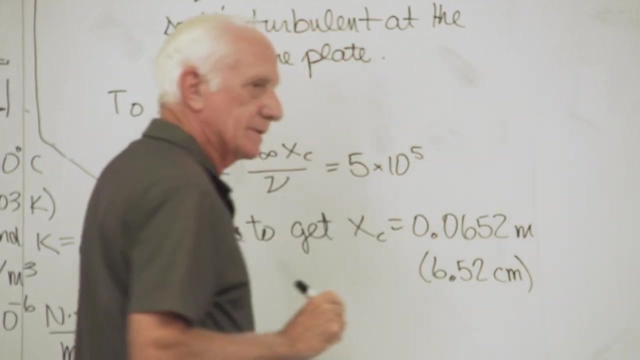 Where does that occur? Reynolds, number Five times 10 to the sixth, 10 to the fifth. Solve to get x sub c. There it is 0.0652.. About six and a half centimeters, Six and a half centimeters. 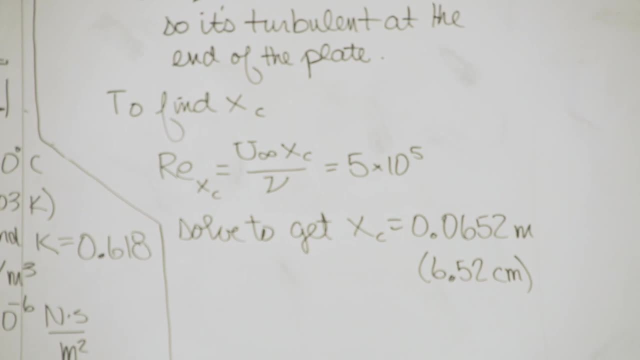 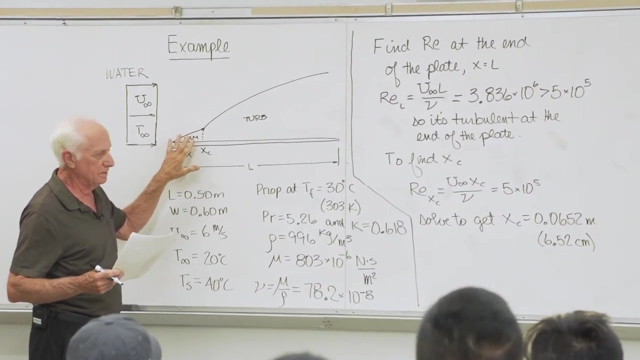 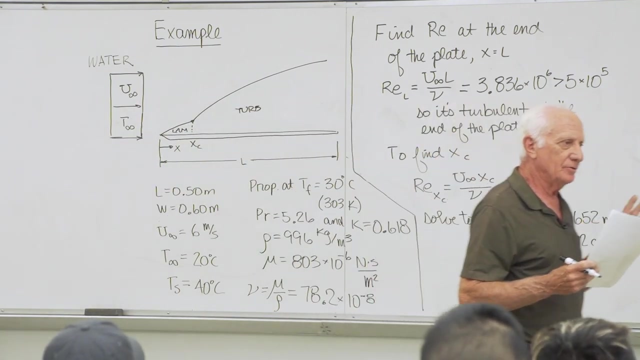 Now, how long is the plate? 50 centimeters. Where does the transition occur? Six and a half centimeters right here, up near the front of the plate. So that's our roadmap. So when you get a problem like this, what you want to do is, first of all: 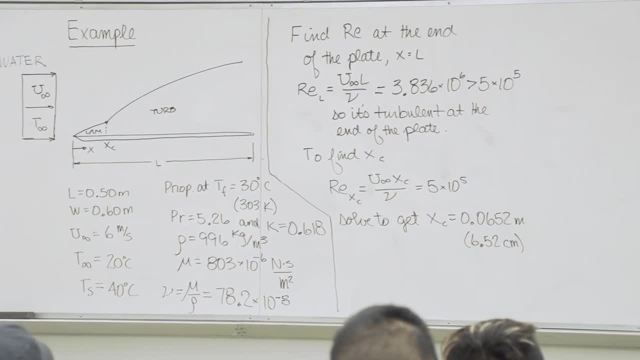 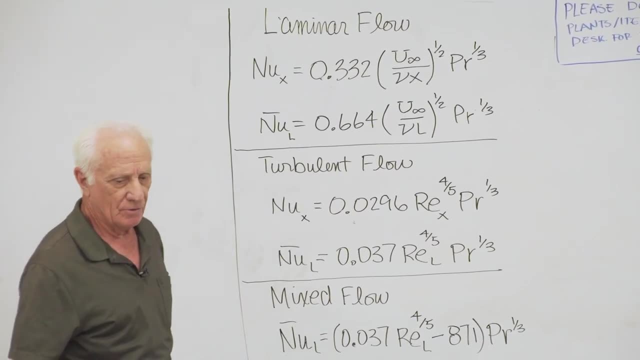 you want to look at the roadmap? What do I have over here? Because I've got a choice- laminar, turbulent, mixed- So I need the roadmap to tell me what I'm going to use over here to solve this problem. 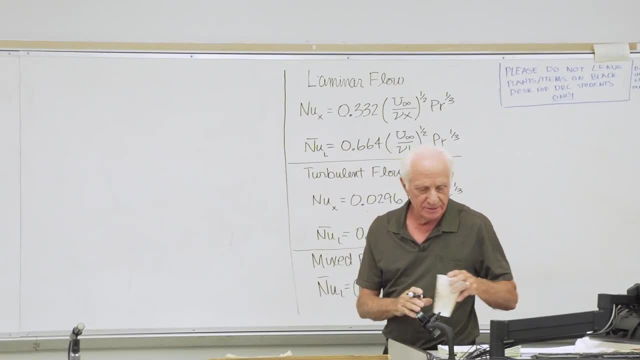 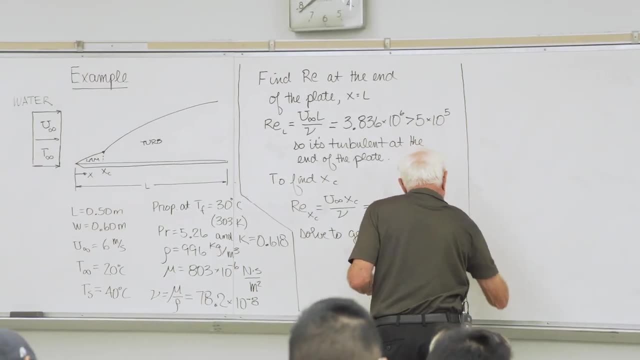 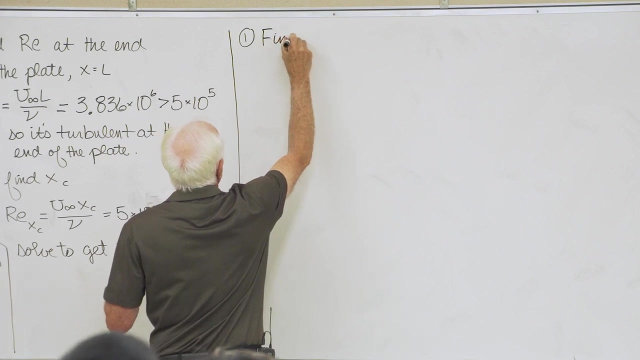 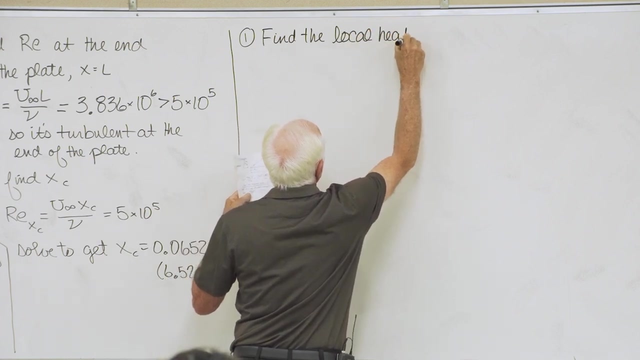 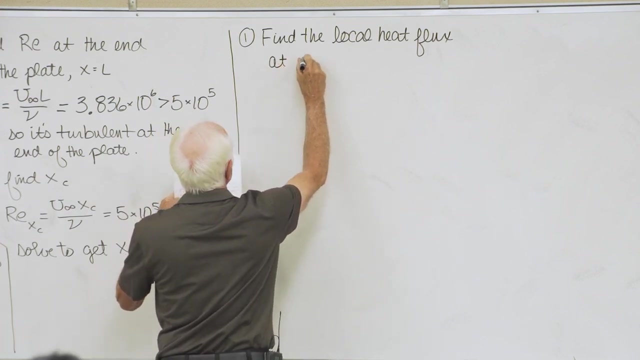 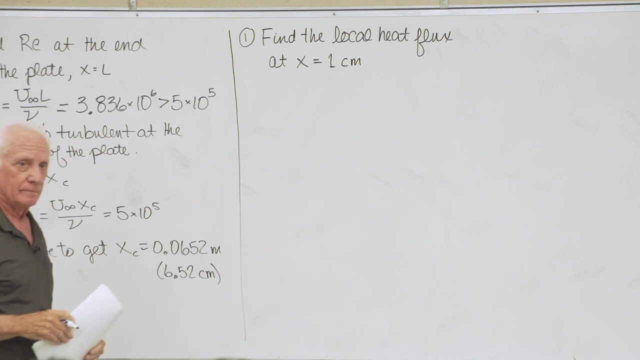 I'm going to solve for various things for this problem. Okay, So number 1.. Here's the first question. Find the local heat flux at x equal one centimeter. Now don't forget where it transisted. it transisted at six and a half centimeters. 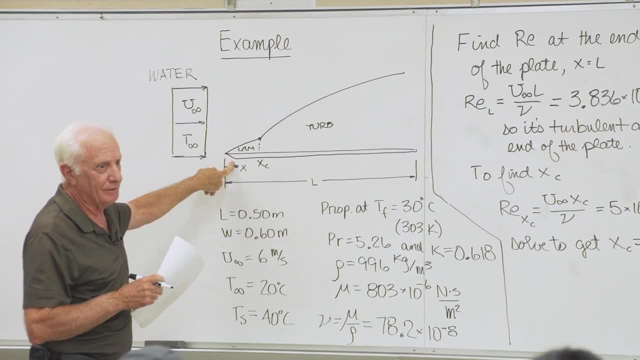 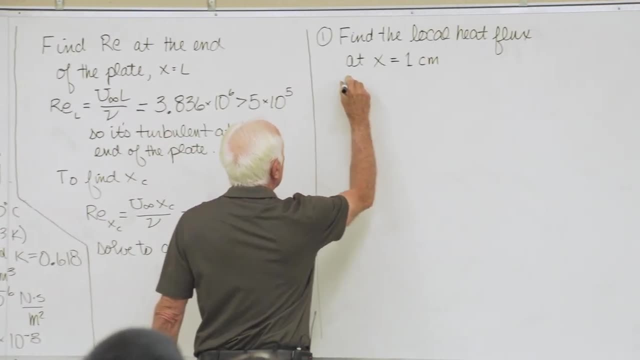 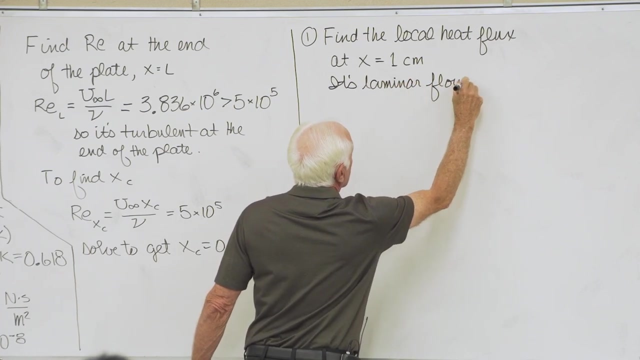 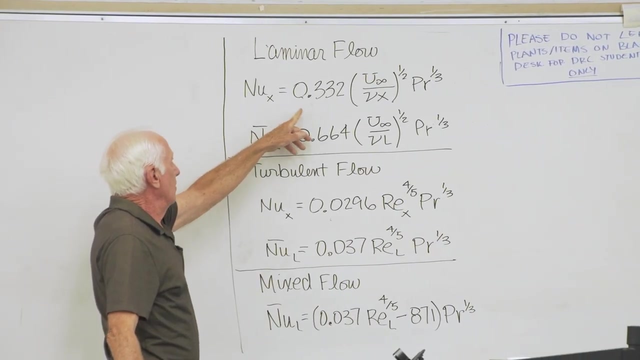 So where my fingertip is one centimeter, conclusion: I'm in the laminar flow regime. It's laminar flow here. Go over to your equations. Do I want the local? That's local. Do I want the average? No, I don't want the average. 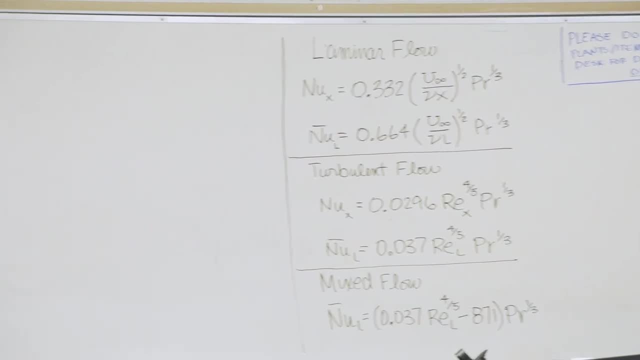 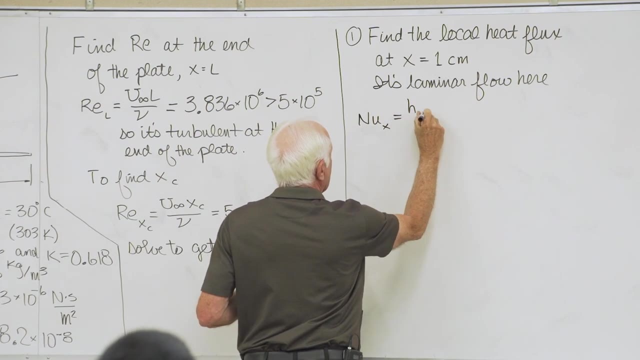 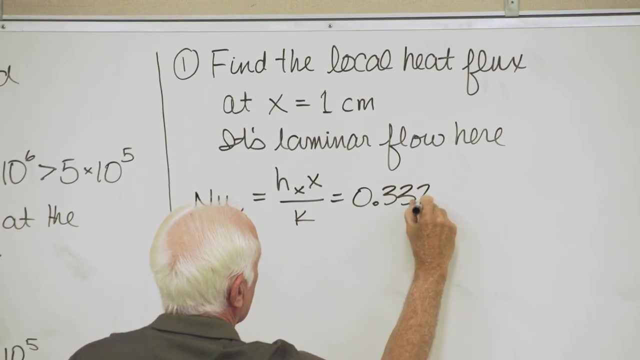 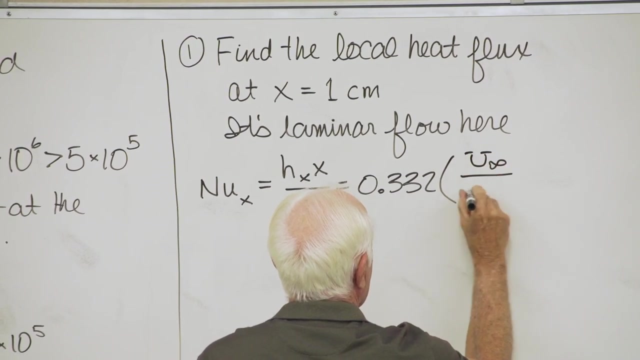 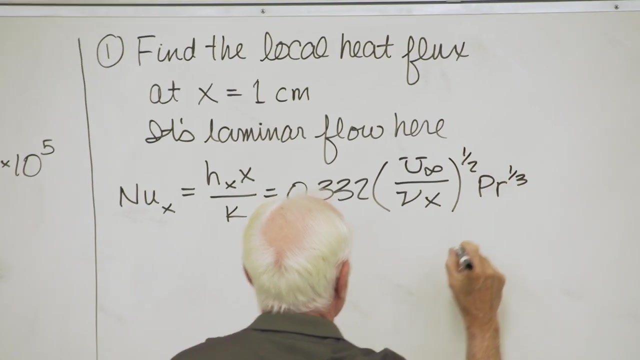 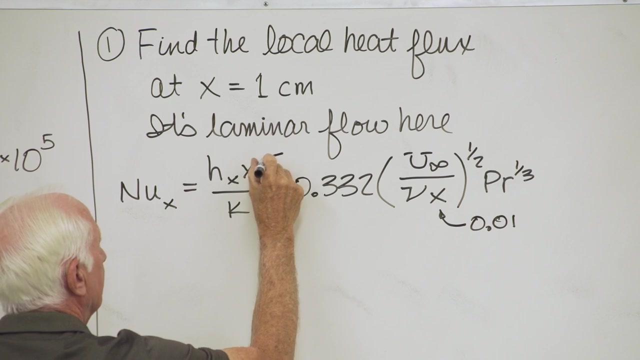 There's my guy right there. What's in this salt number Hx? Well, let's write it down: Hx: Laminar flow u infinity over nu. x one-half Prandtl to the one-third. What's x One centimeter? 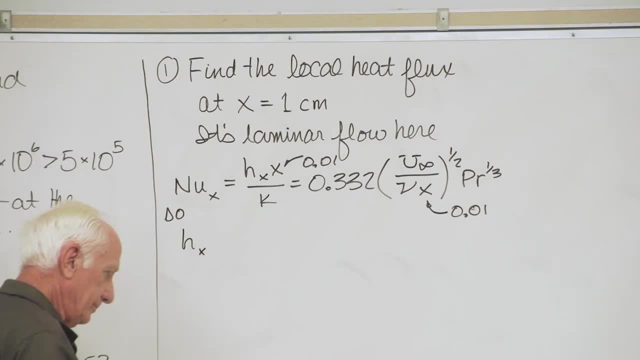 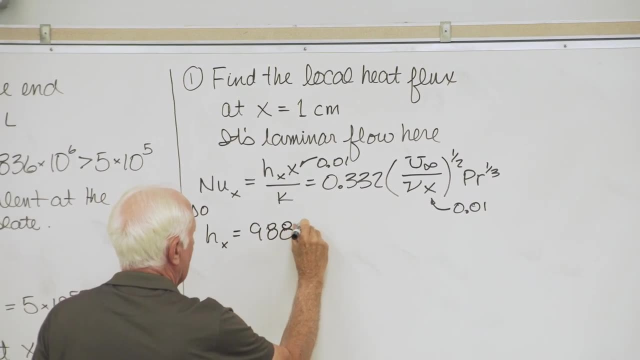 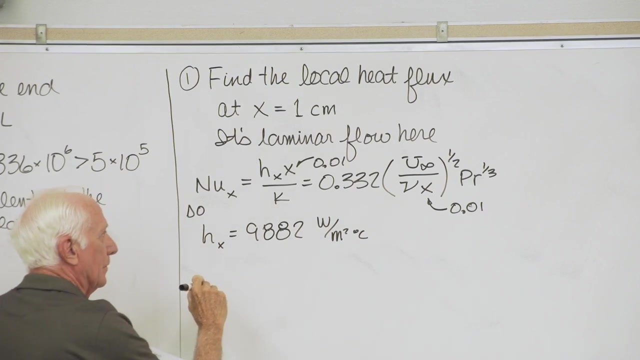 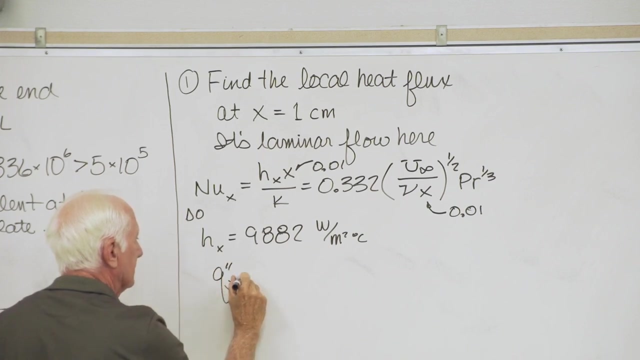 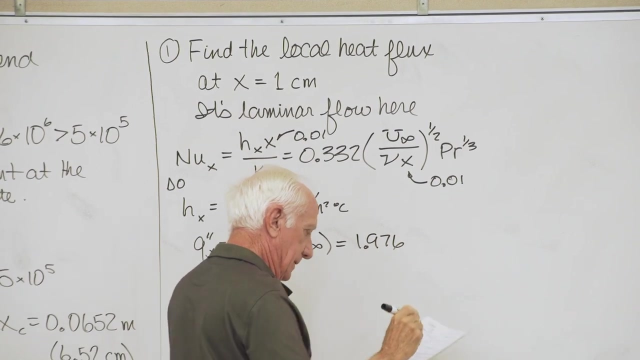 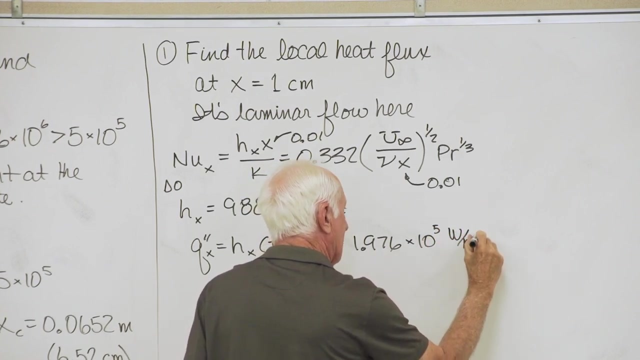 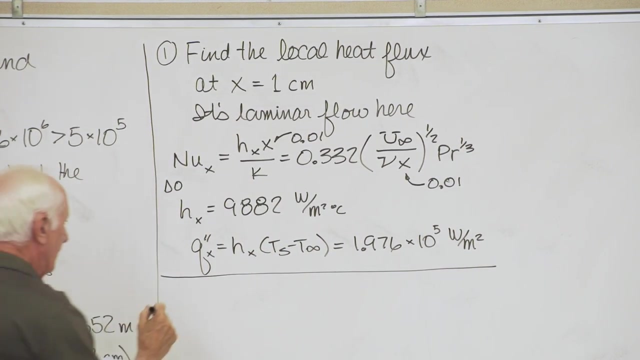 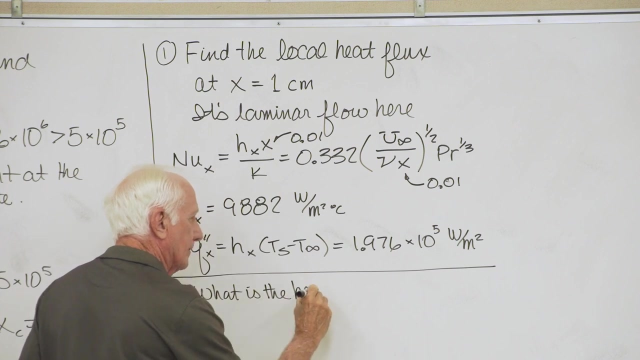 Solve for Hx 98, 82.. Heat flux. Heat flux q, double prime, Local x. There it is 1.976 times 10 to the fifth watts per square meter. Number 2.. Number 2,: what is the heat transfer? 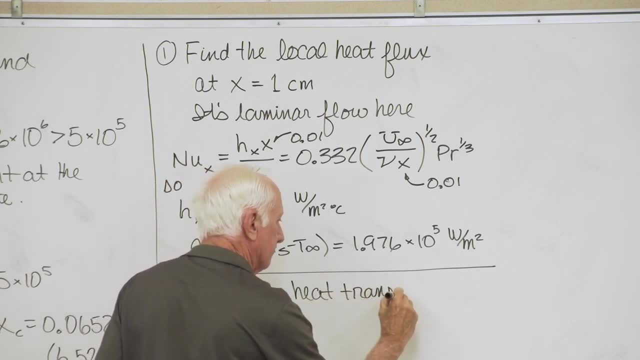 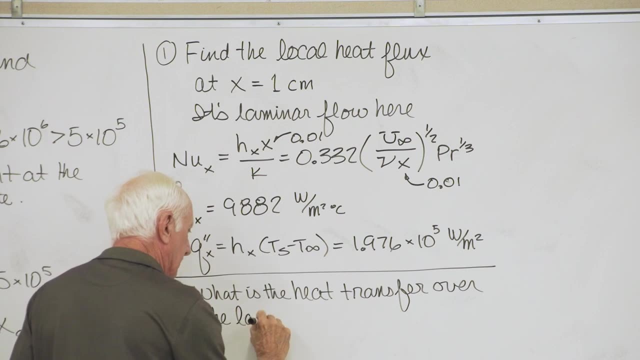 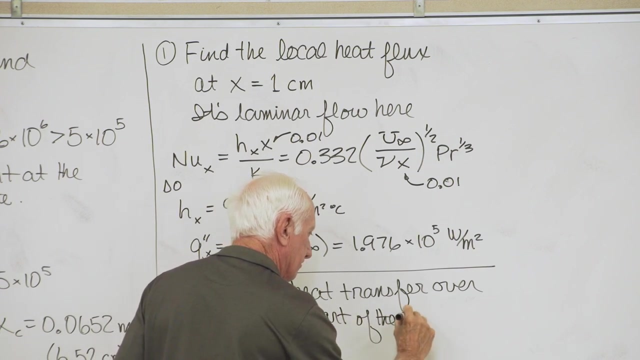 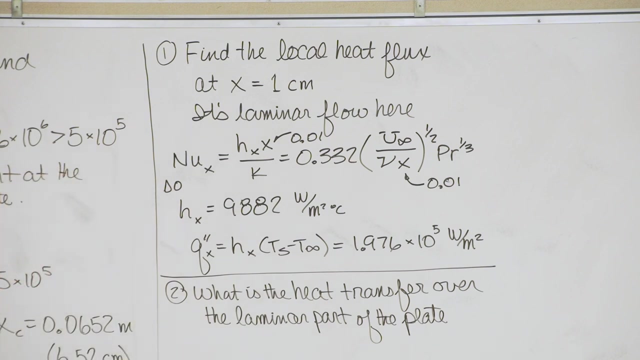 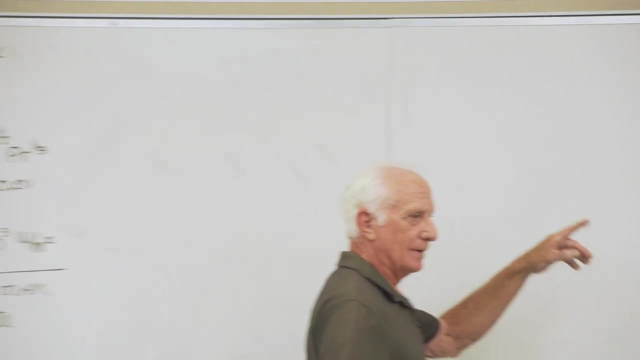 over the laminar part of the plate. 1.716.. 1.716?, 1.716?, 1.716? 1.716? Not the local, I want the whole heat transfer over the laminar part of the plate. 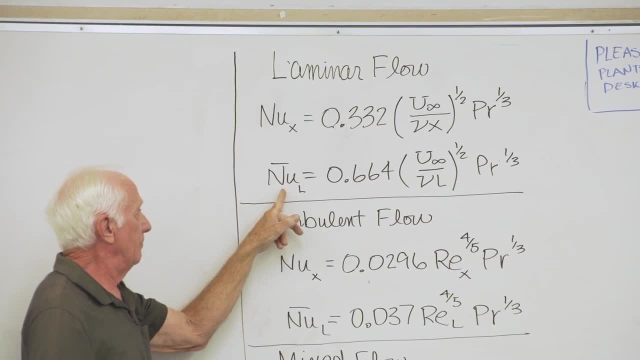 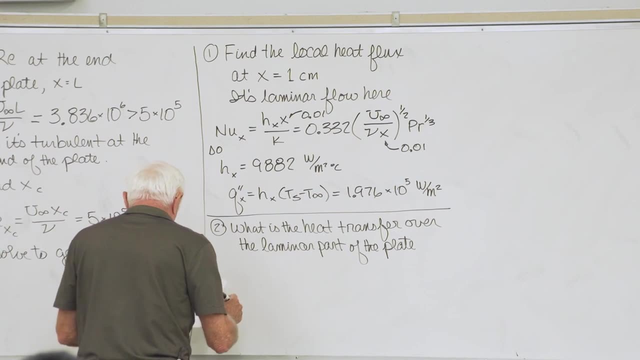 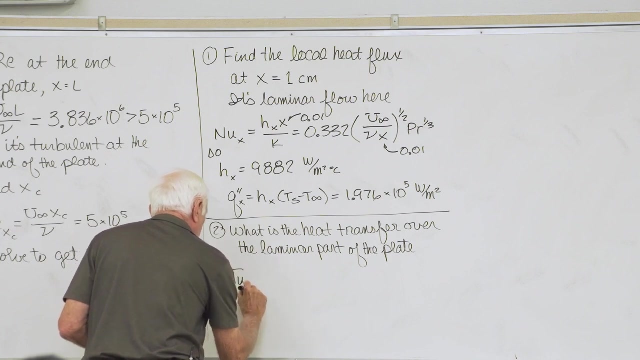 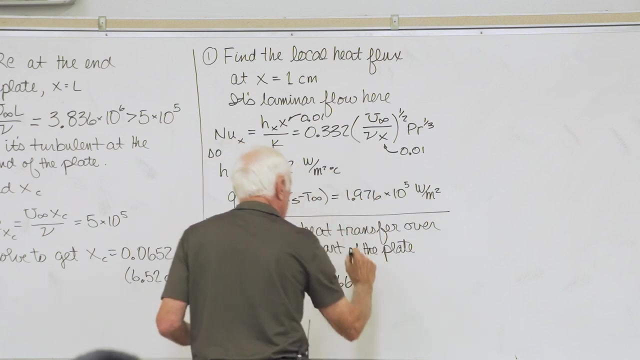 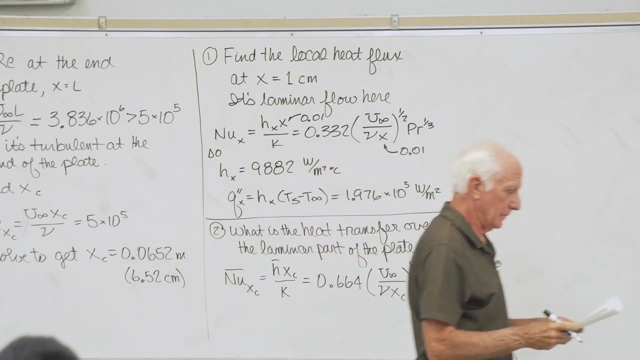 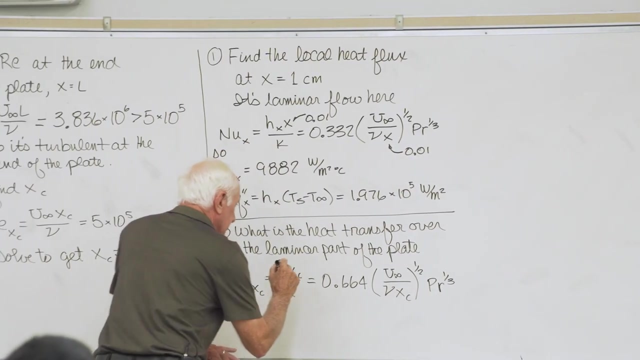 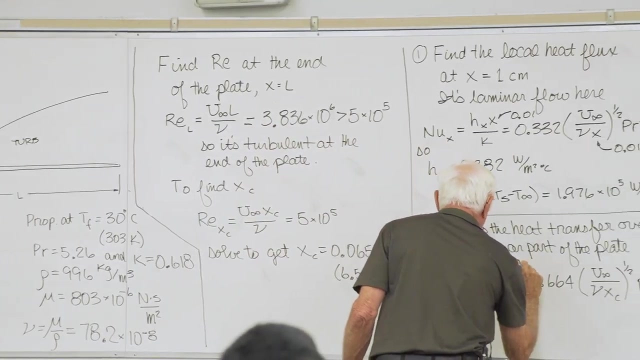 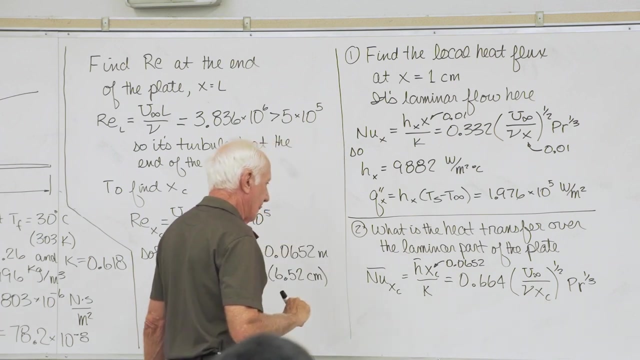 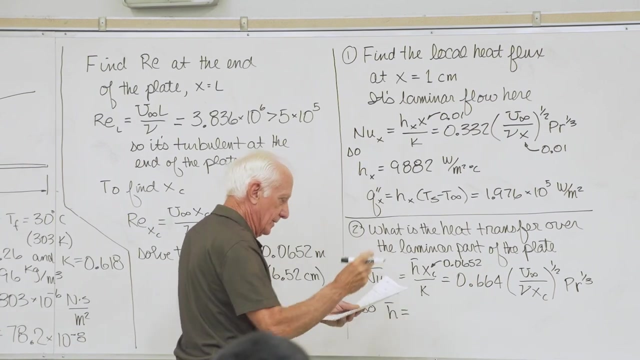 Laminar Average H. that's what I want to use. okay, So my no-salt bar 0.664.. Same thing here: X of C right there. So H bar. You know everything there. 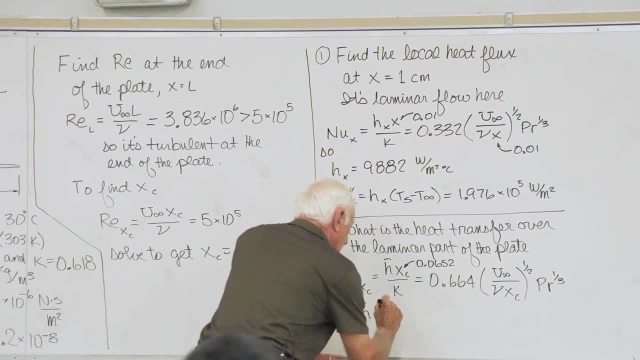 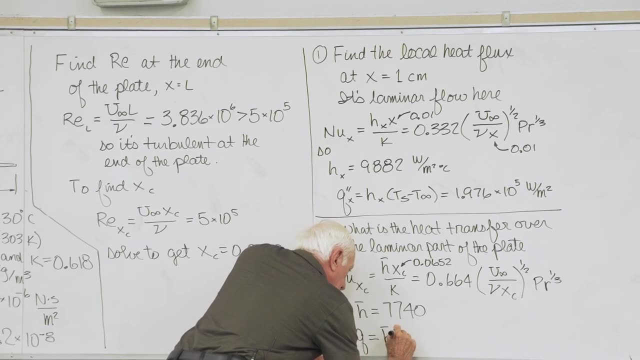 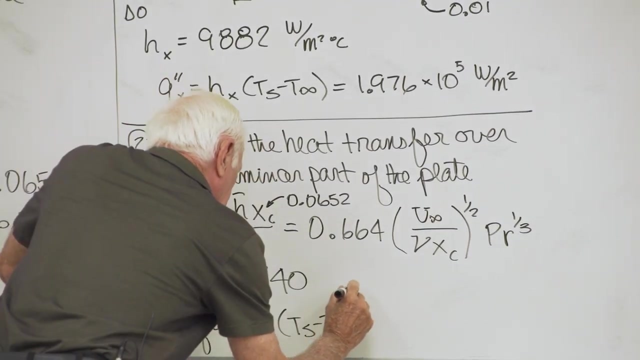 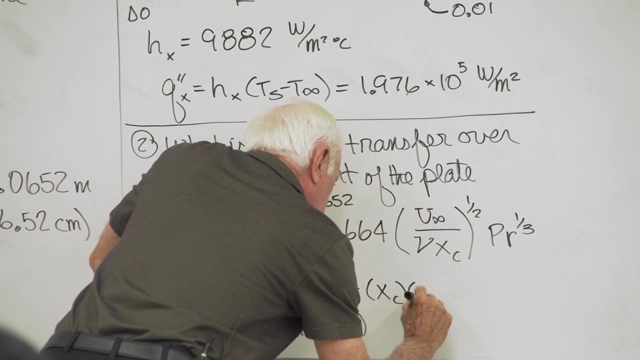 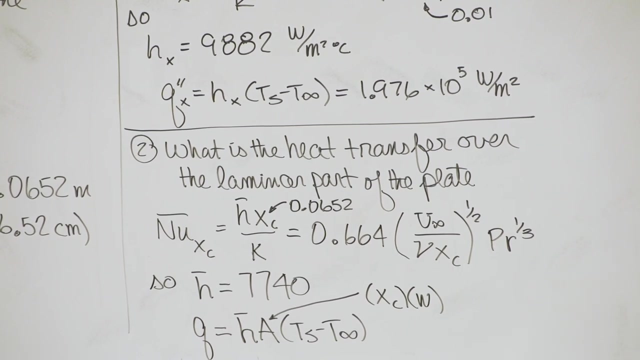 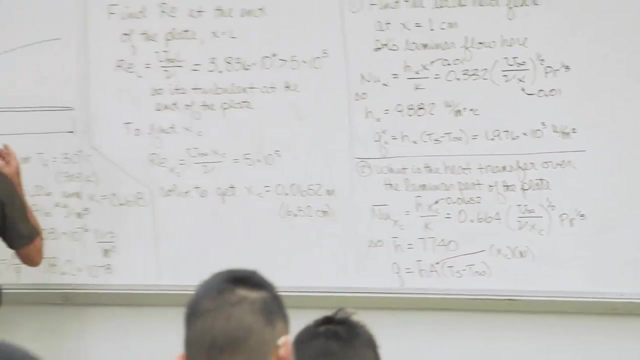 H bar- H bar. H bar 7740.. Q over the laminar part of the plate: H bar times that particular area: T S minus T infinity. That area is X of C times W. There's the homework I told you last time. the rule right hand, left hand. 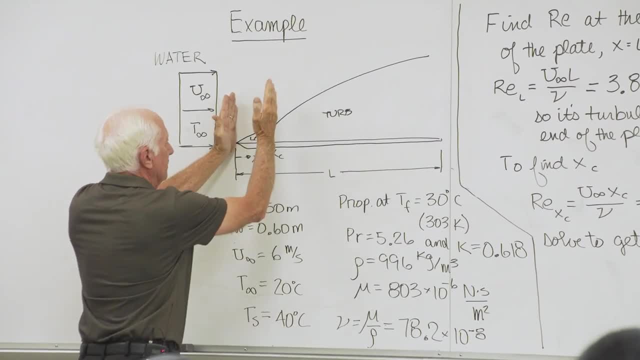 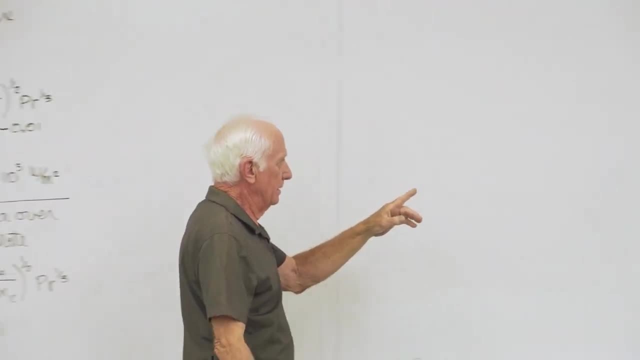 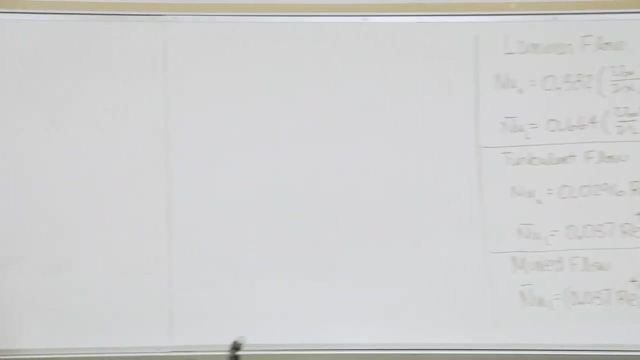 Where do you want to find the heat? transfer My right hand to my left hand. Where's my left hand At X of C? In this equation, what's L? Don't put 50.. See, people will say: oh yeah, no, no, L is 50.. 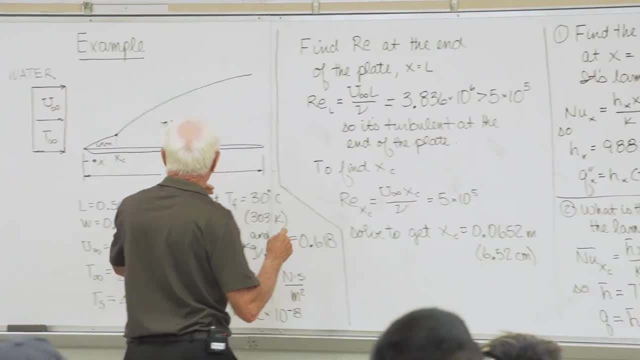 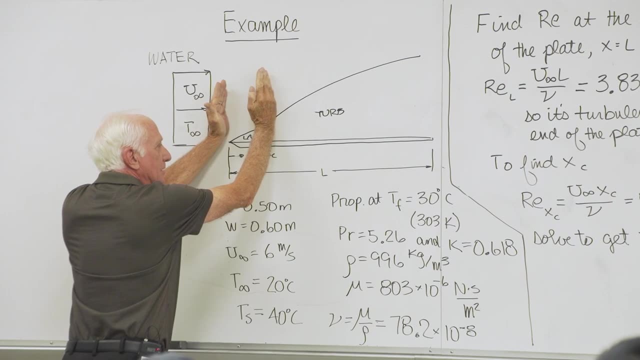 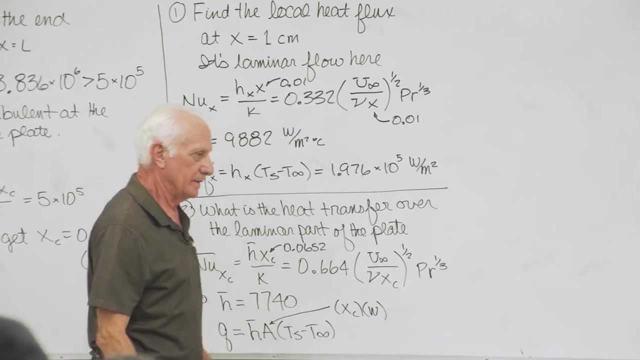 Oh no, it's not. It's where my right hand is again: Left hand, right hand. I want the average convection coefficient between my two hands. My right hand is at X of C, So that's why I put X of C in here. 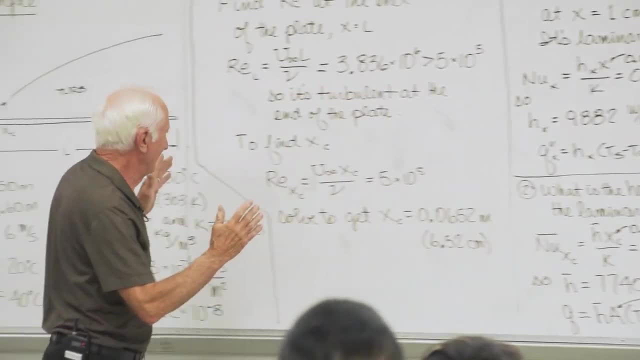 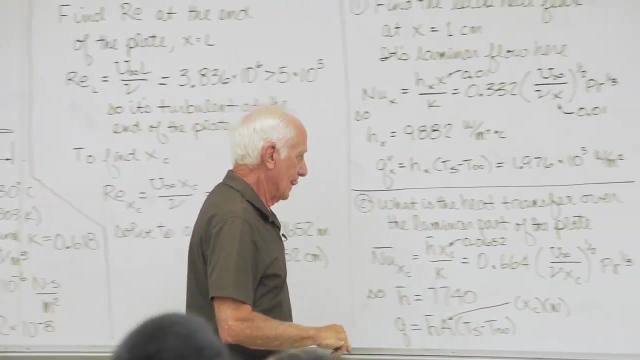 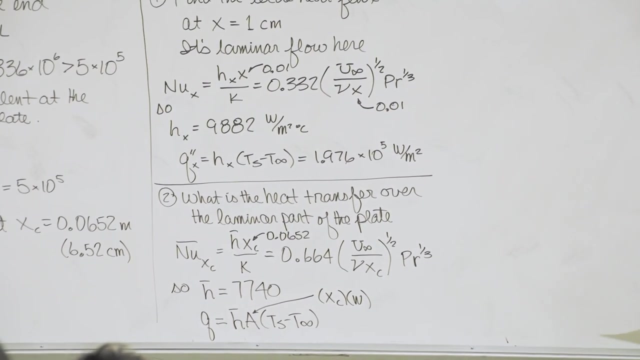 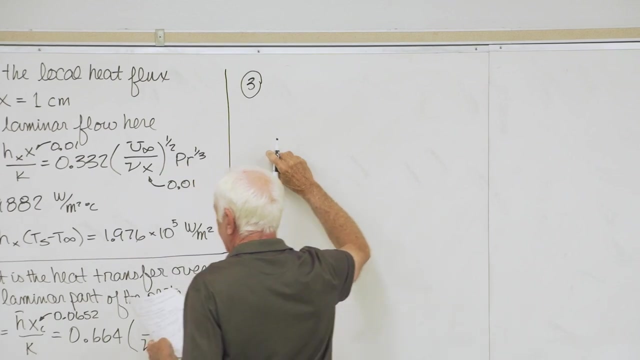 Oh, and then the area between my right hand, left hand. Don't take the whole area, No, it's this. distance times W: 0.6. W. Now let's do part 3.. Find the heat transfer over the whole plate. 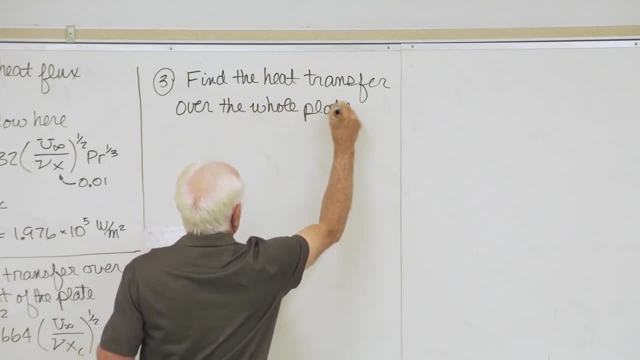 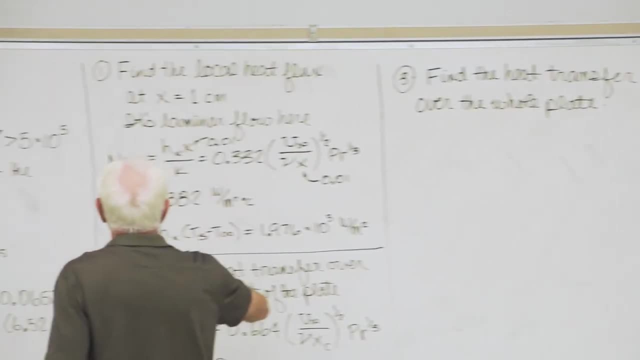 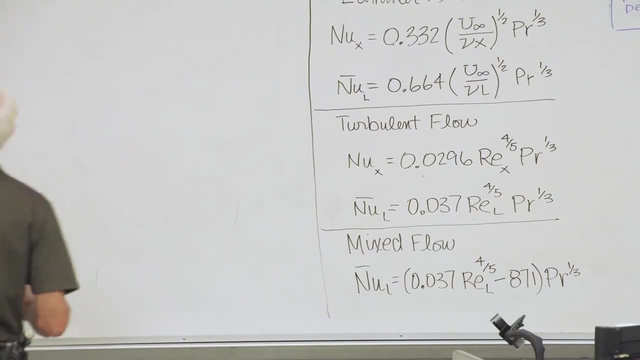 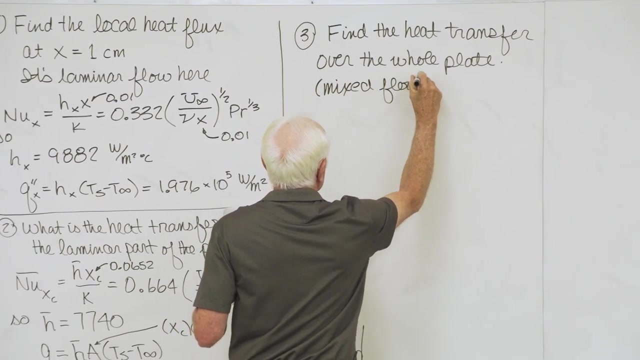 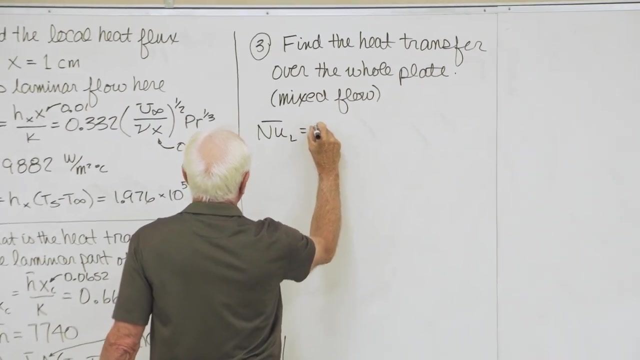 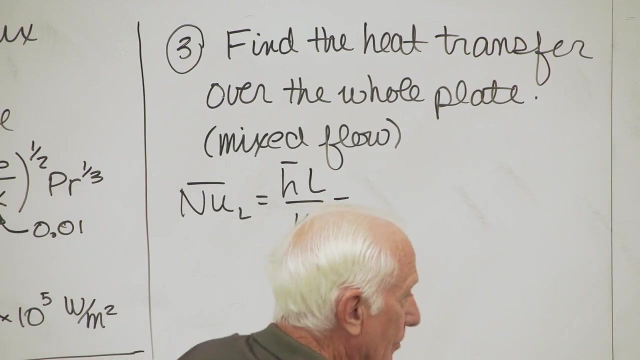 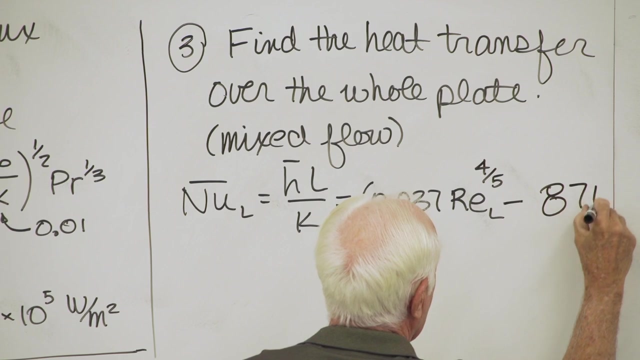 Okay, Roadmap said what Roadmap said: mix flow. Okay, Okay, Mix flow, Okay. So no salt bar L Is equal to H bar L over K: 0.037.. Reynolds L to the four-fifths minus 871.. 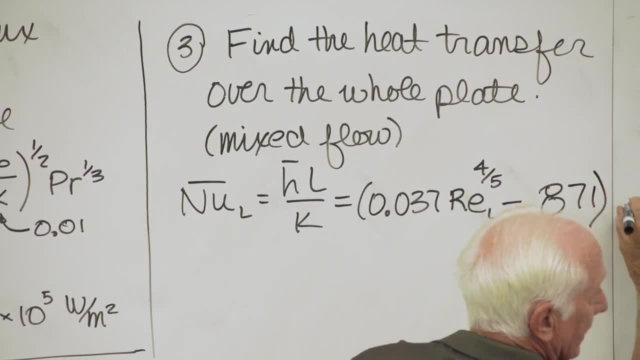 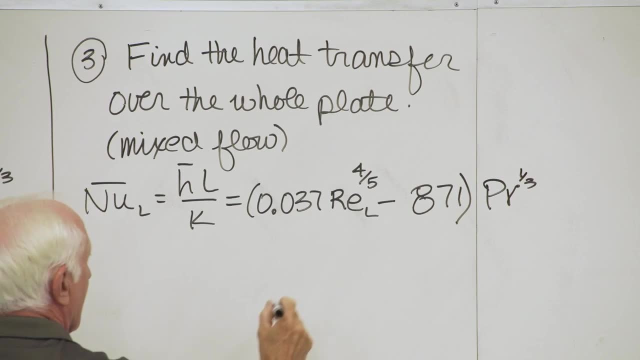 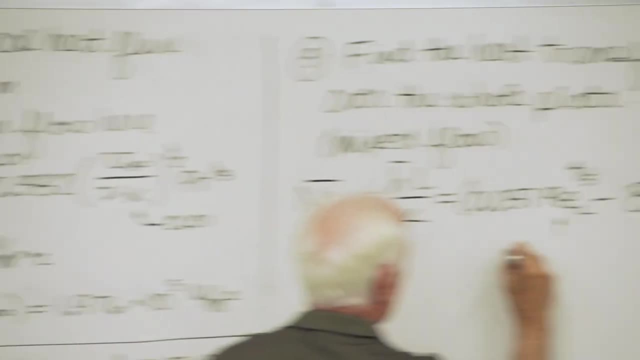 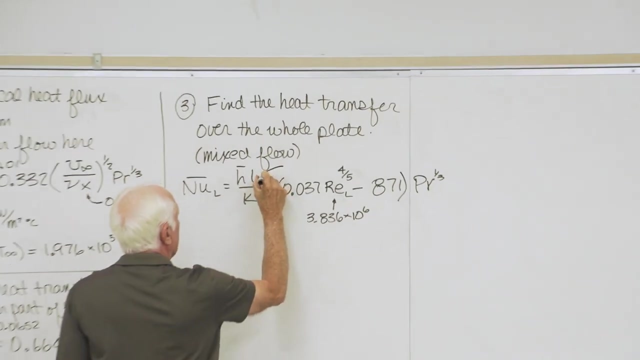 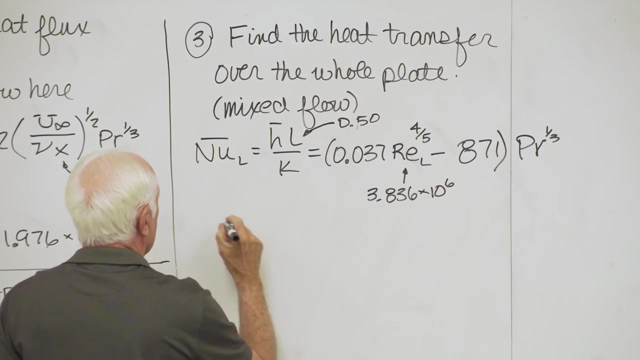 Crandall to the one-third: Okay, That Reynolds number at the end of the plate: 3.836 times 10. to the sixth: That L 50 centimeters From that I get H bar, Okay, Okay. 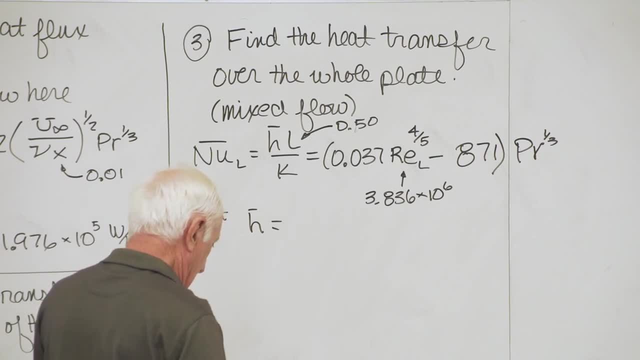 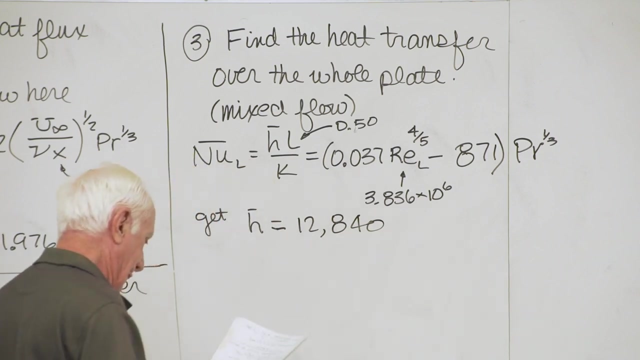 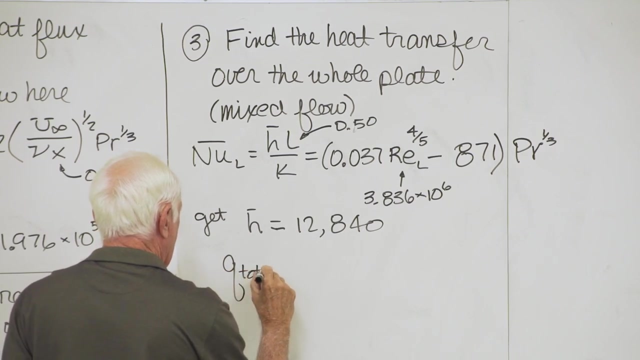 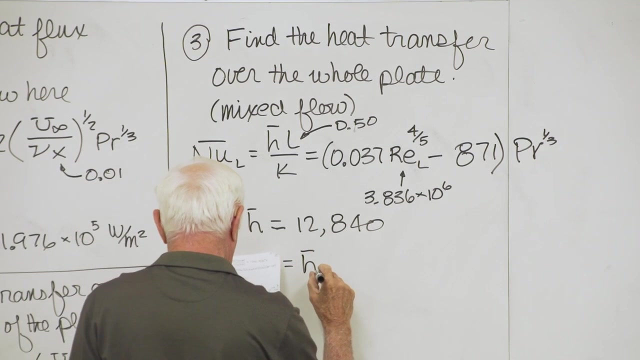 Over the whole plate. Okay, we've got there. it is 12,840.. Over the whole plate: H bar 0.037.. Okay, Over the whole plate: H bar 0.037.. Bar Times the area. 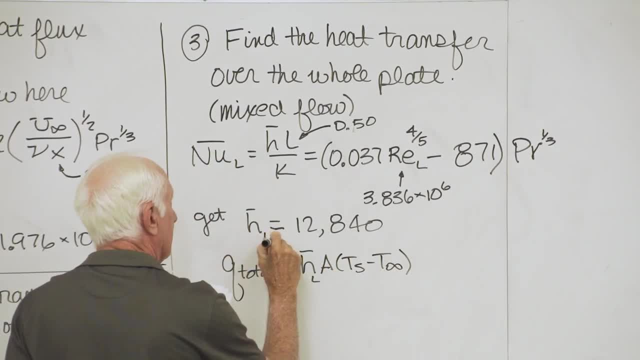 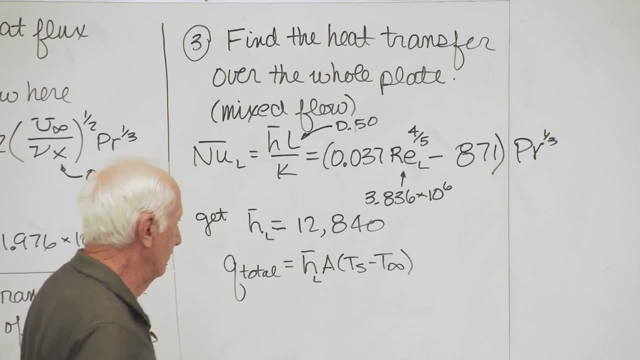 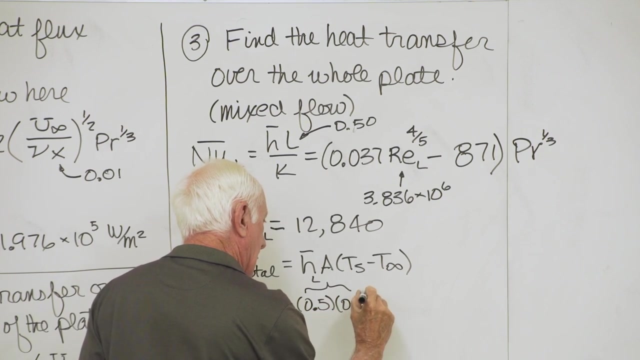 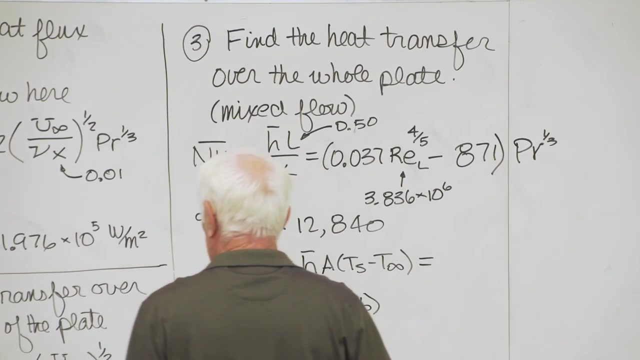 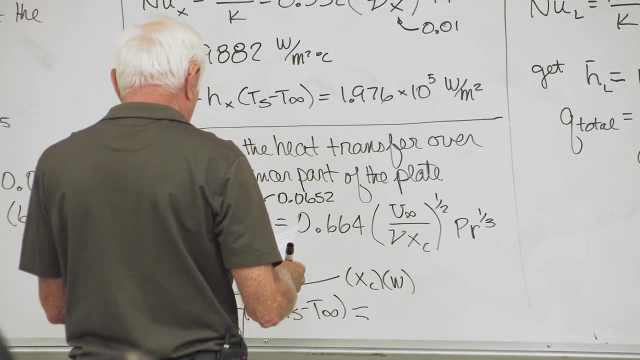 〔. The area, the whole plate. worship 0.5 by 0.6.. 0.5, well, I'll put it here: Whole plate. We didn't get queued on here, sorry about that. That was over the laminar part of the plate. 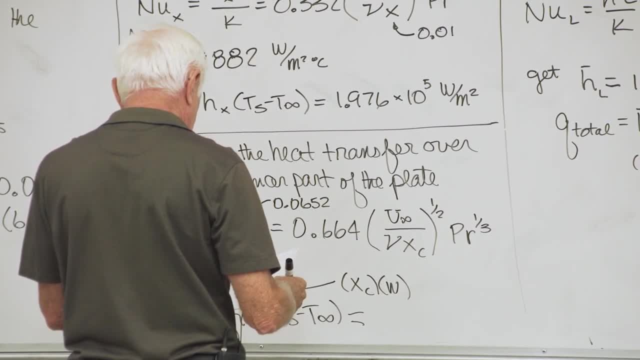 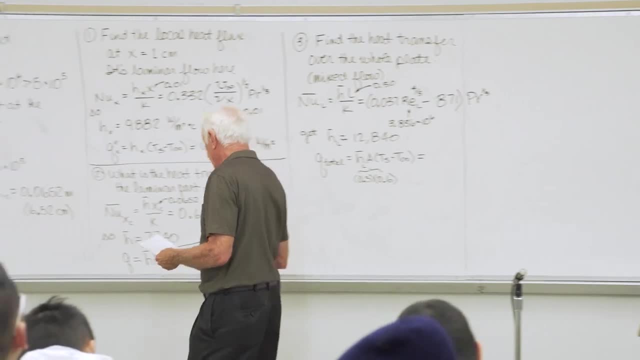 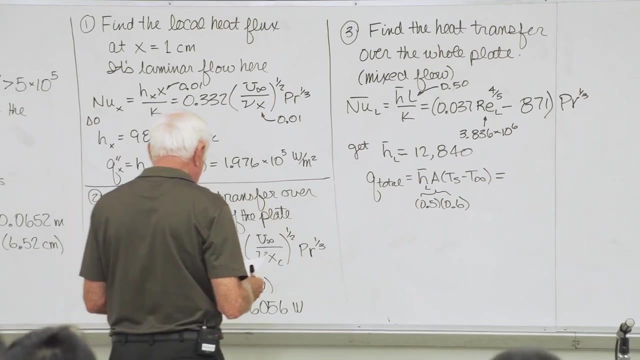 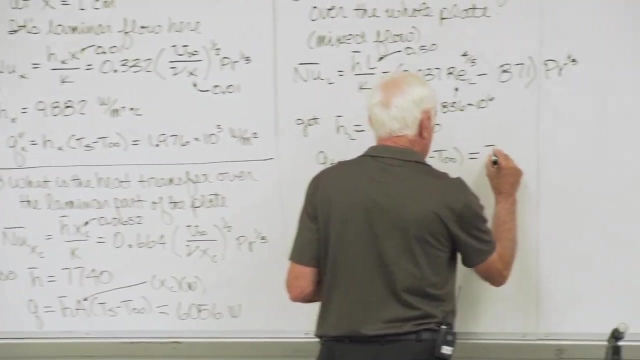 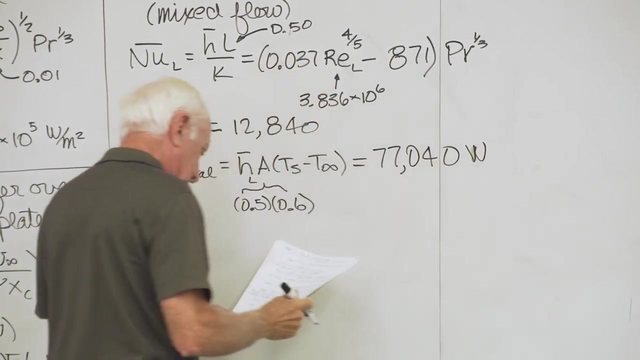 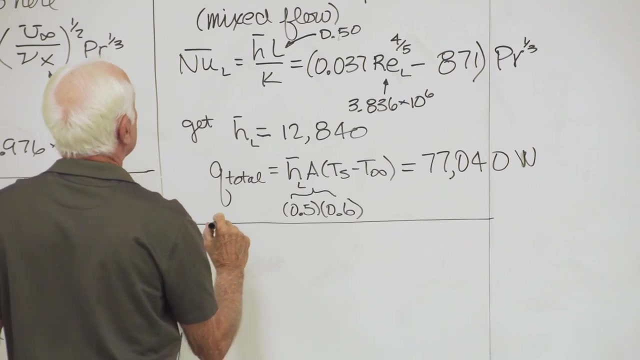 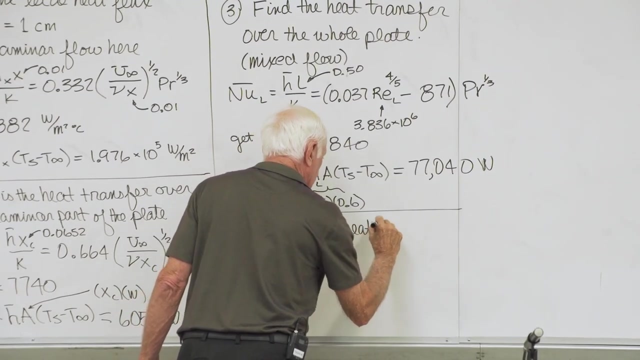 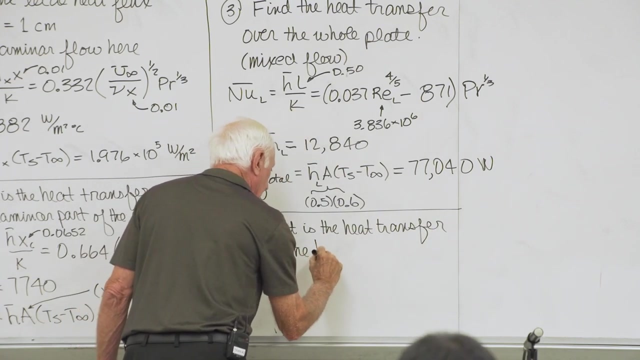 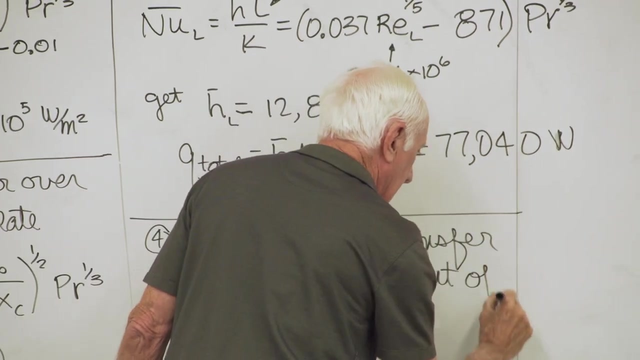 Let's see what my queue was there. Oh here, okay, 6056.. Okay, back over here This guy here. queue total: 77040.. Watts, What is the heat transfer? Okay, Over the turbulent part of the plate. 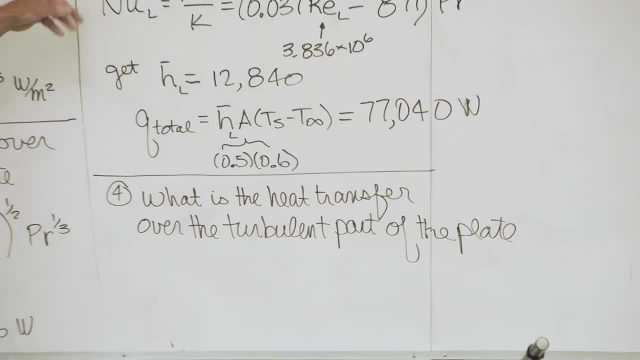 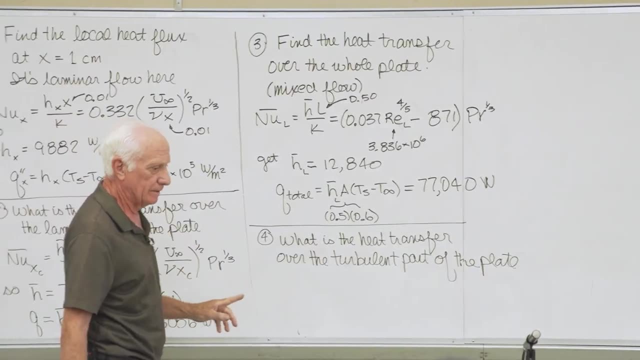 So part 3 over the whole plate, part 2 over the laminar part of the plate, part 4 over the turbulent part of the plate. Now, what you don't want to do is you don't want to do this. 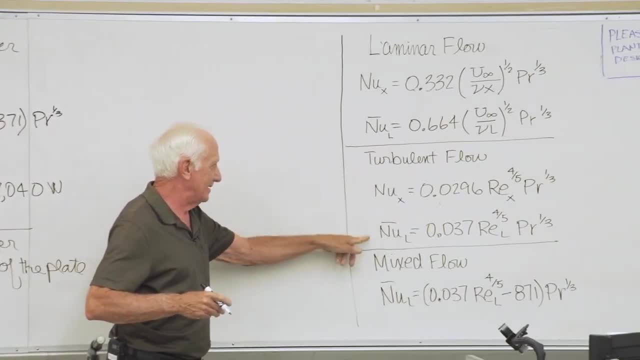 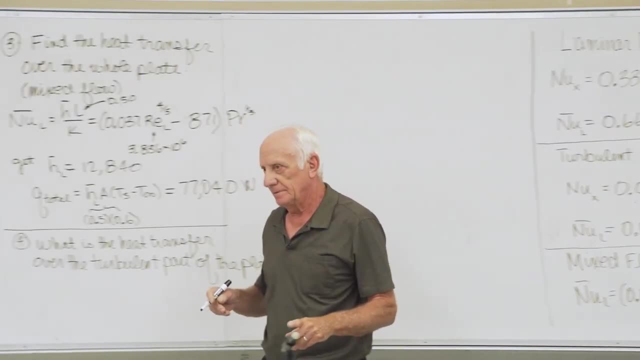 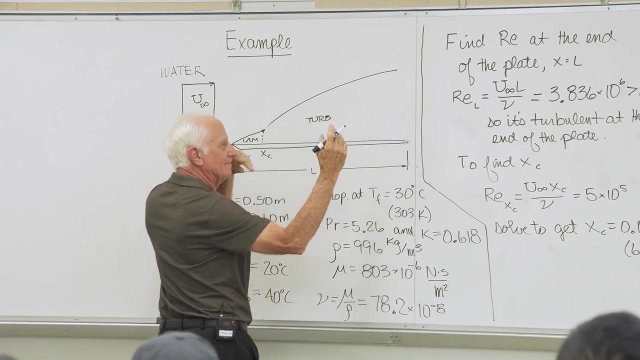 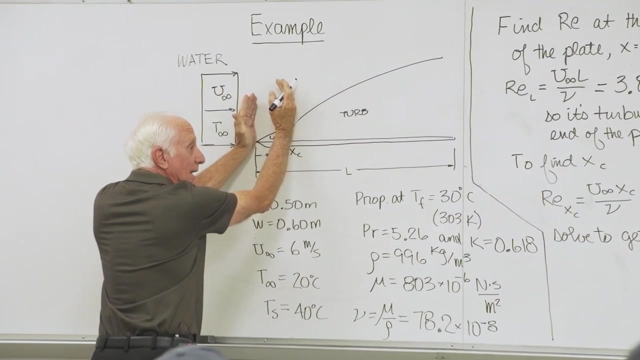 What you don't want to do is say, oh yeah, turbulent, got it right there, the average turbulent. No, no, The heat transfer- right hand, left hand, heat transfer over the whole plate, minus the heat transfer over the laminar part of the plate, gives you the heat transfer over the turbulent part of the plate. 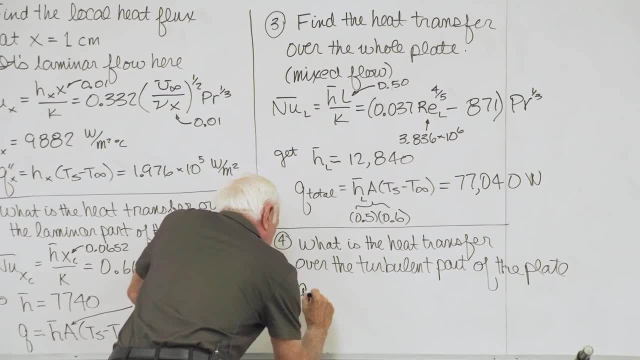 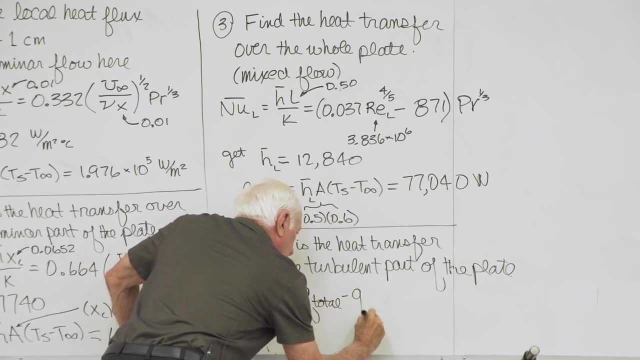 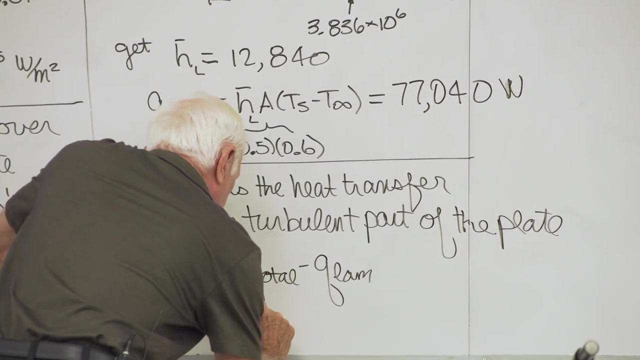 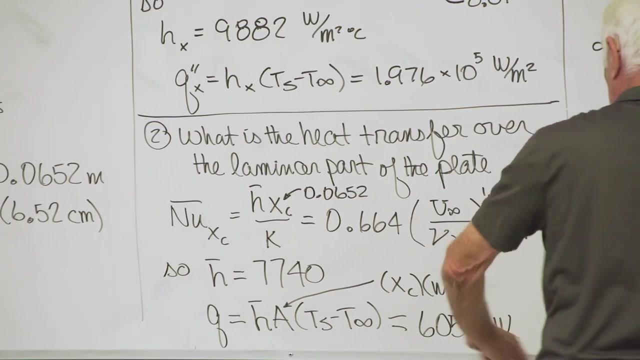 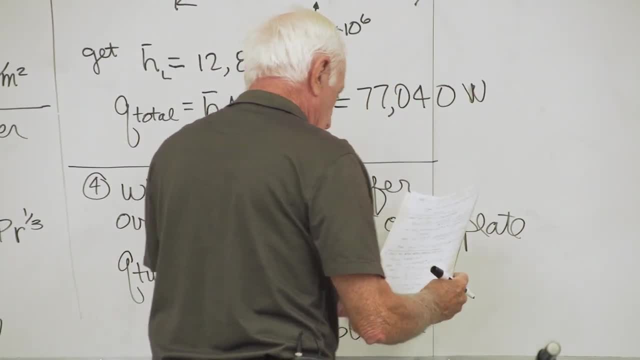 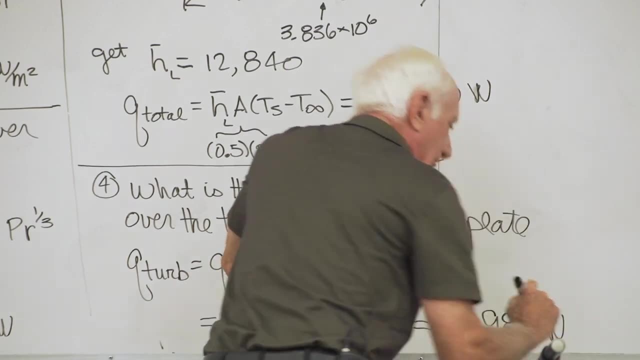 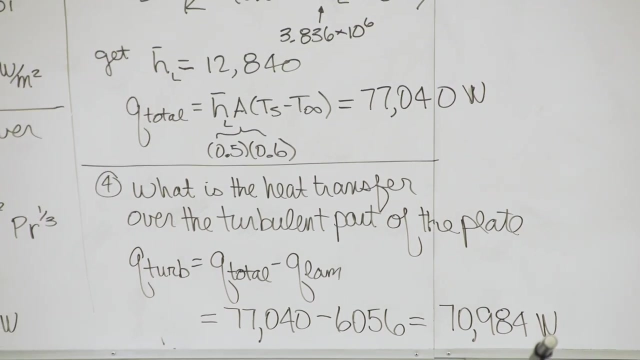 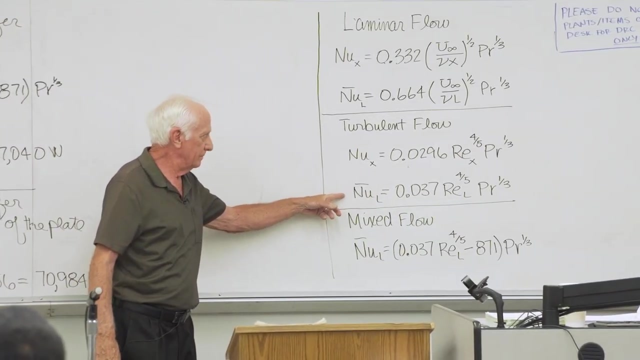 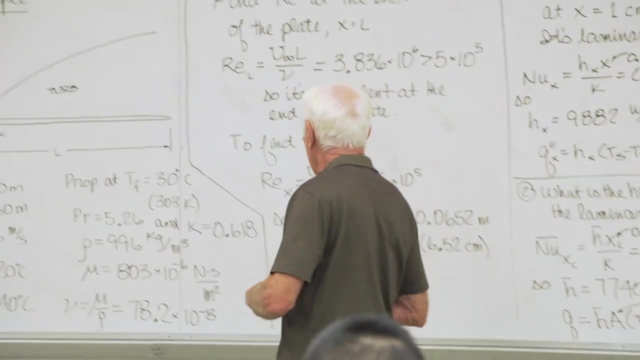 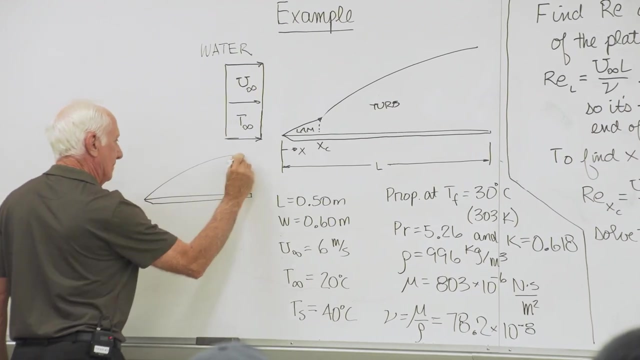 So over the turbulent part of the plate, 70,984.. So you say, well then, when can I use him? You didn't use him in this problem. No, I didn't use him because this wasn't the problem. Was it turbulent from x equals zero. 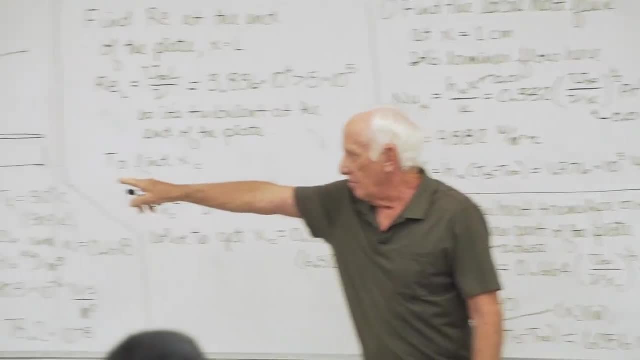 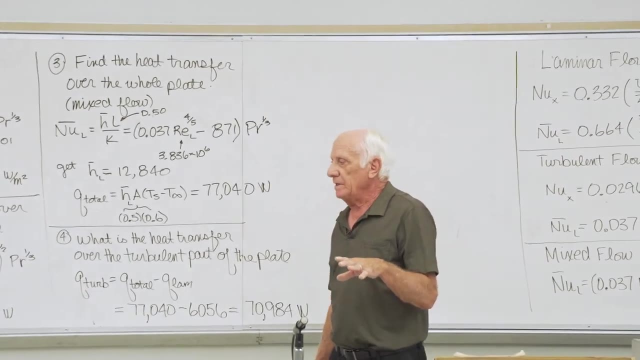 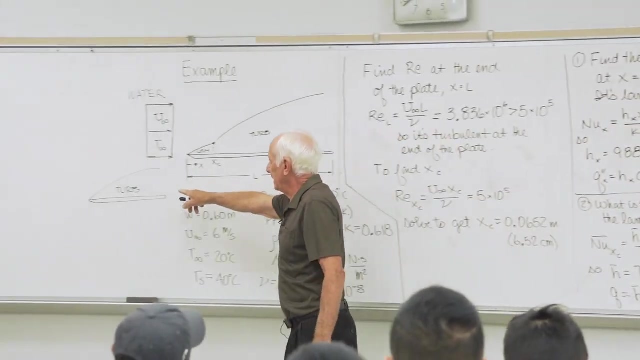 No, If that was my problem over there, turbulent Now. if the problem said for homework or an exam, if it says, by the way, assume the flow is turbulent from the leading edge. That's my picture: Turbulent from the leading edge. 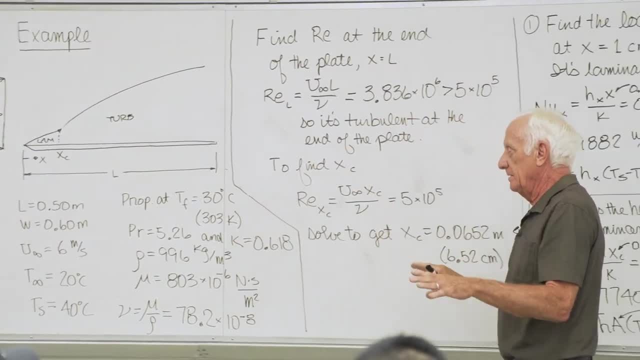 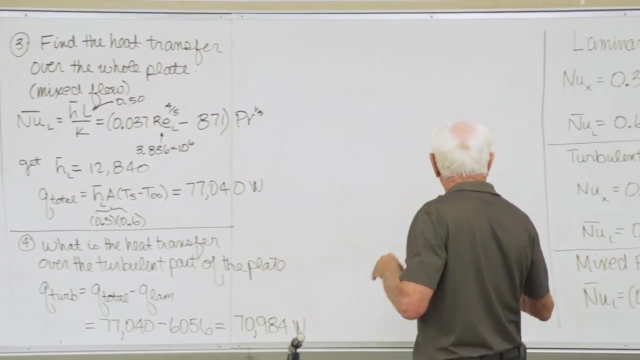 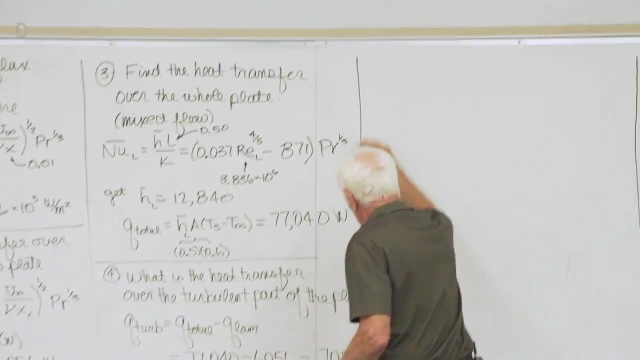 My problem didn't say that. It said nothing. If it says nothing, assume it starts out laminar and it may or may not transist to turbulent flow. Okay, So that's why we didn't use this guy. If someone says: oh, you know what? 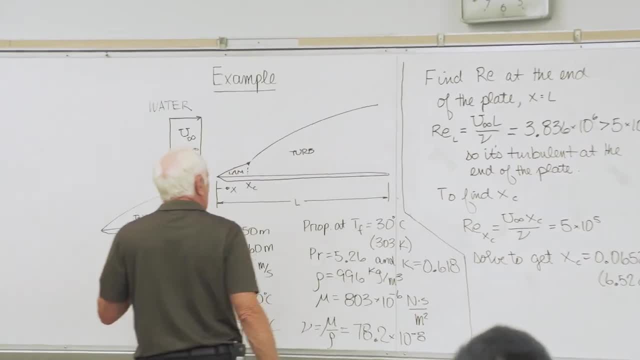 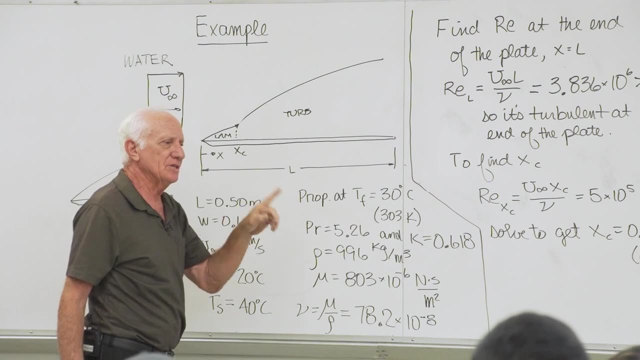 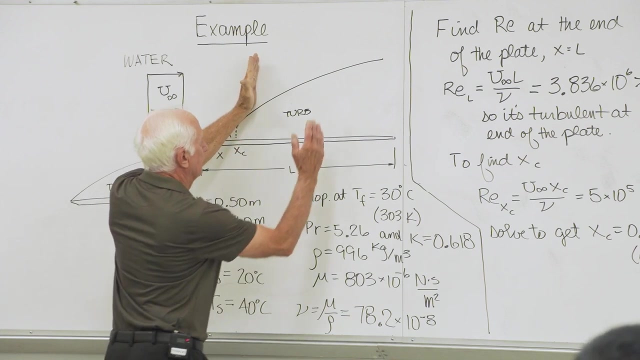 This is what I want. I want you to find out how much heat is transferred. This is x equals 50.. How much heat is transferred from 20 centimeters to 40 centimeters? 20 to 40 centimeters, Here's 20.. Here's 40.. 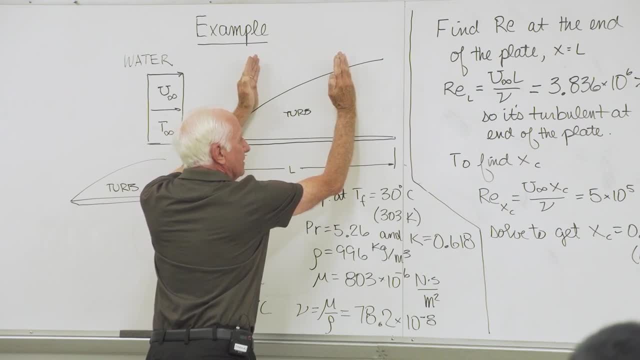 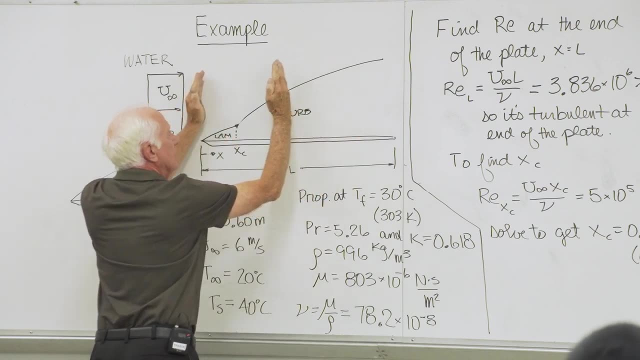 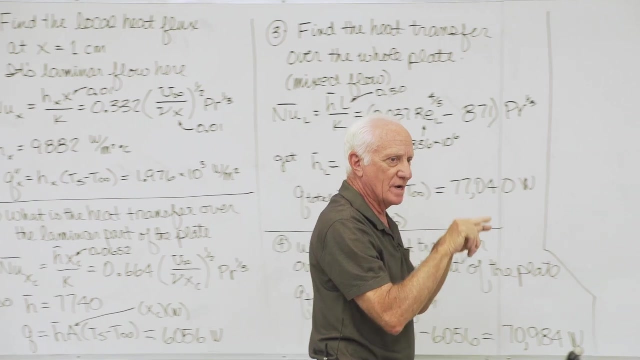 It's in the turbulent range, Got it? How do I find it? Okay, Find the heat transfer from zero to 40. Then find the heat transfer from zero to 20. And subtract them. Subtract them. That'll give you the heat transfer from 20 to 40.. 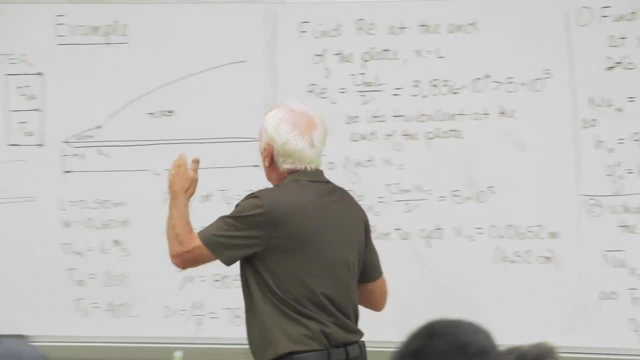 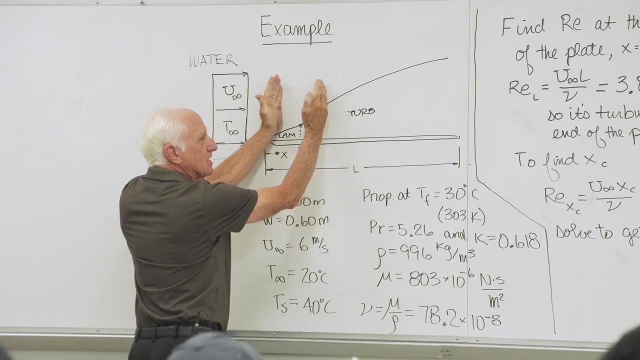 So I don't care where your right hand or left hand is, I'm going to be over here at x equals 2. And I want to go from x equals 2 to x equals 10.. How much heat transfer there? Okay, Find from zero to 10.. 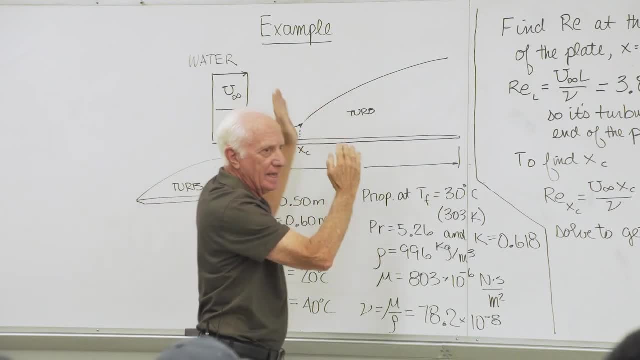 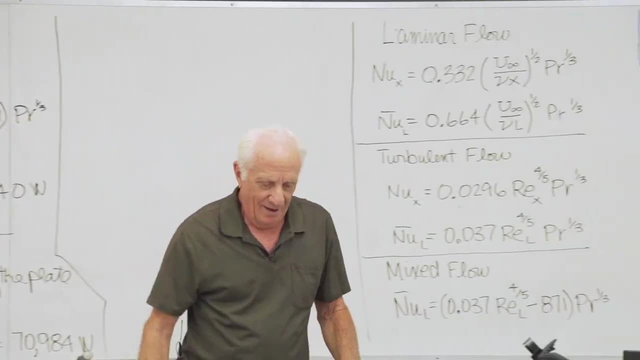 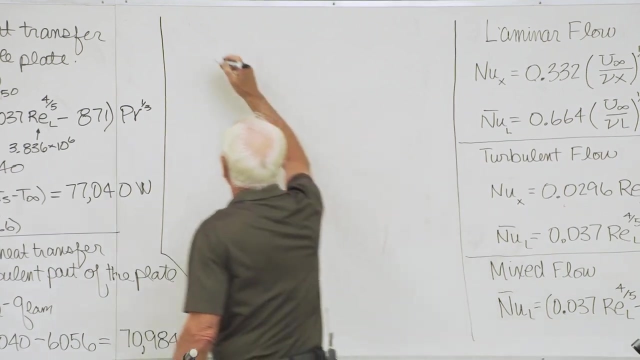 Subtract zero to 2. And that gives you 2 to 10.. Anywhere a band Question You okay, No, Okay, Okay. Now there's another rule. This is a rule. This is called the 10 percent rule. 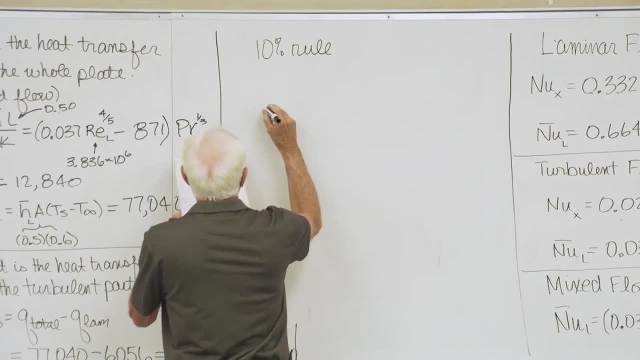 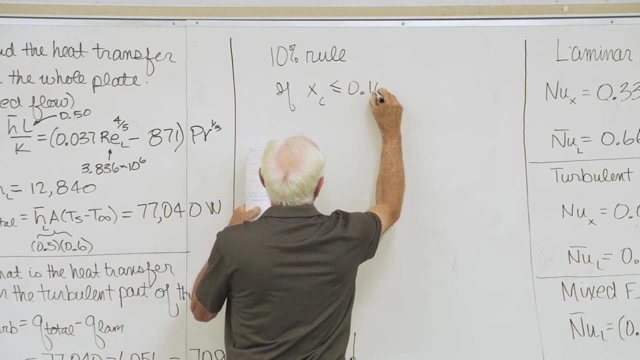 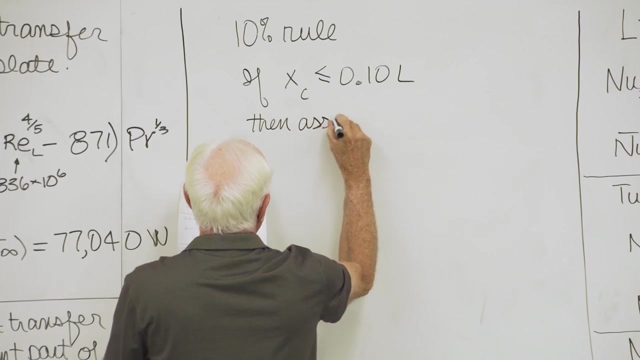 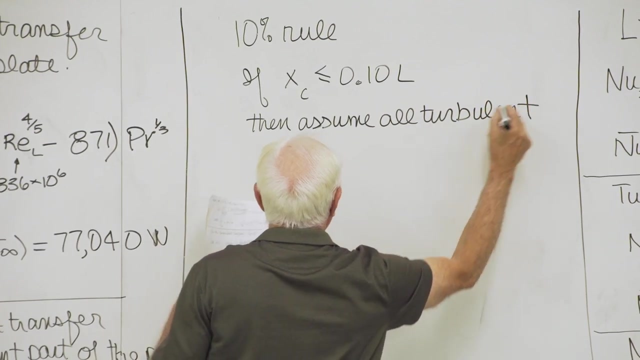 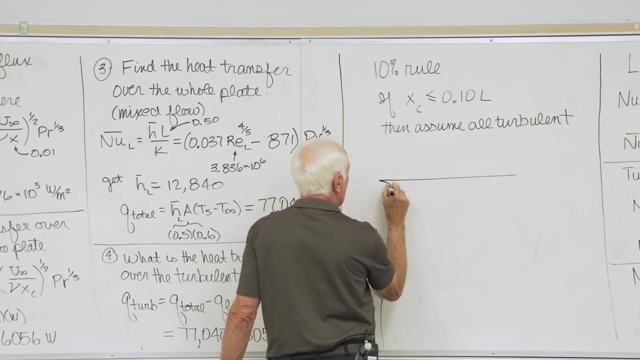 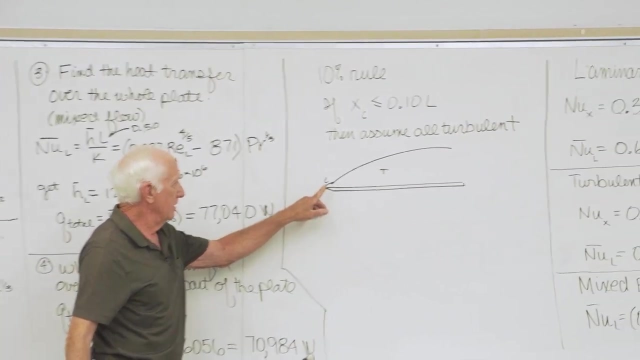 This is what it says. If x sub c is less than or equal to 10 percent of L, then assume all turbulent. Well, why can we assume it's all turbulent? Well, look at the picture, If the transition, the transition, occurs way down here. 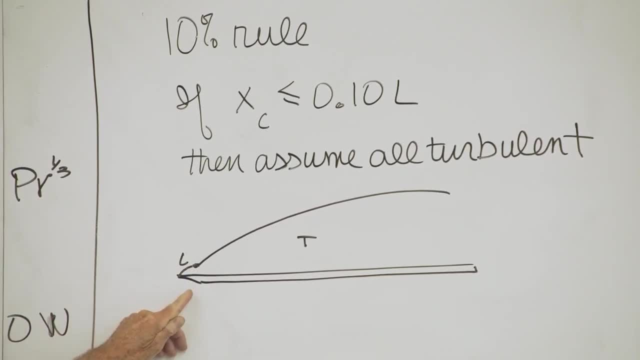 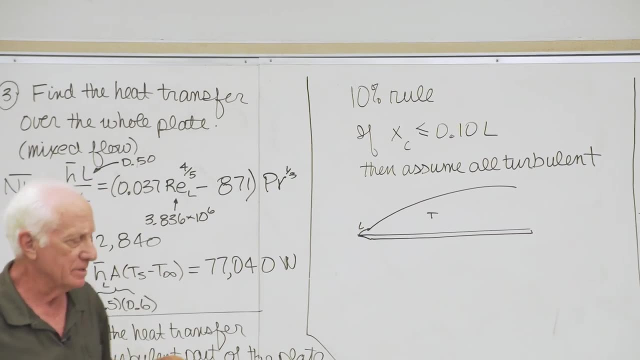 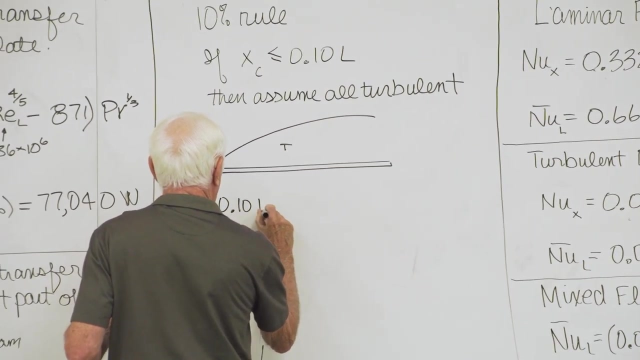 close to the leading edge. it looks like it's almost all turbulent flow over the plate. Yeah right, So we assume it is. It makes life easier and it's a pretty reasonable answer. So let's take our problem here. Our problem here: 10 percent L. 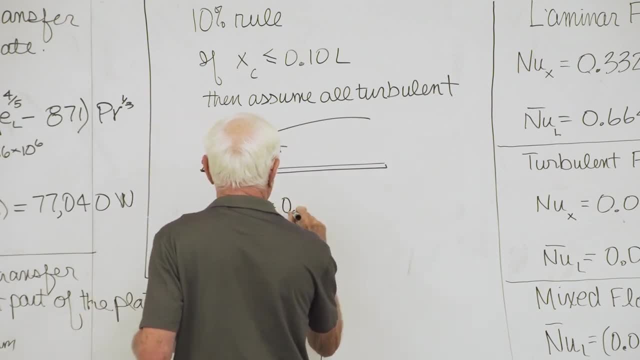 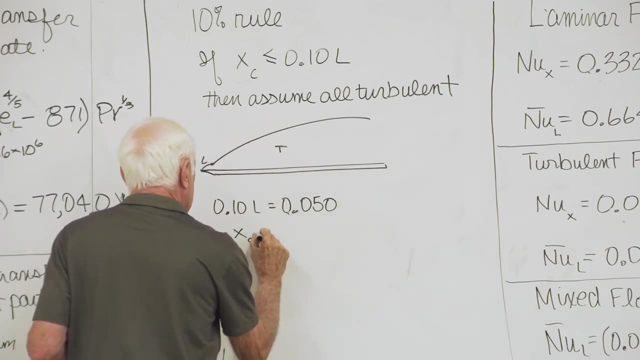 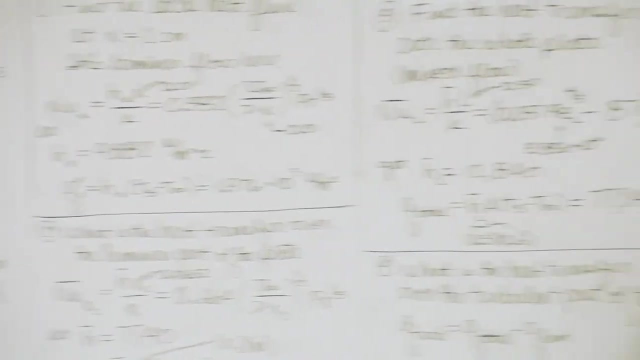 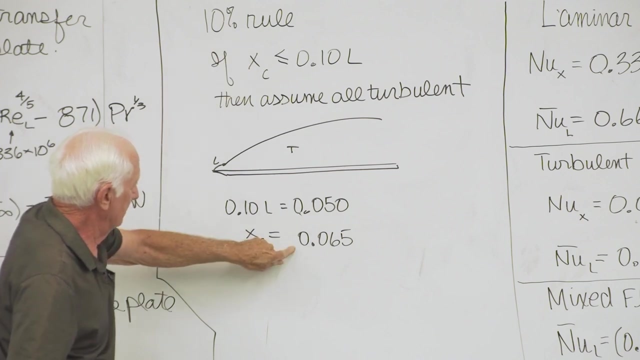 L is 0.5, so it's 0.05.. Okay, x sub c. we found out there it is 0.0652.. And you ask the question: is x sub c less than that Is 0.065, less than 0.050?? 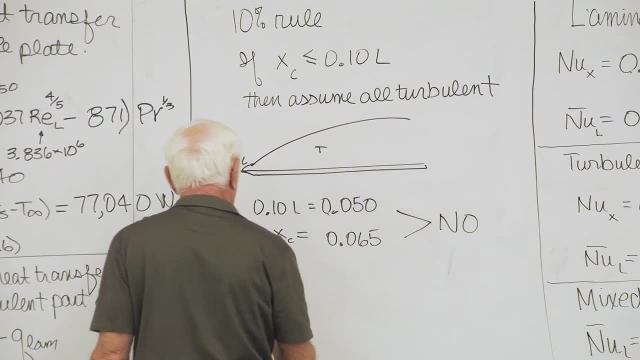 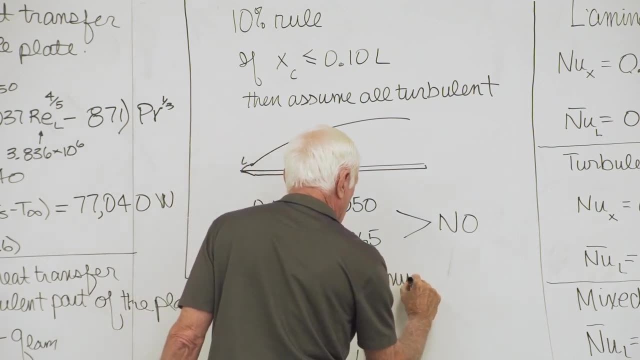 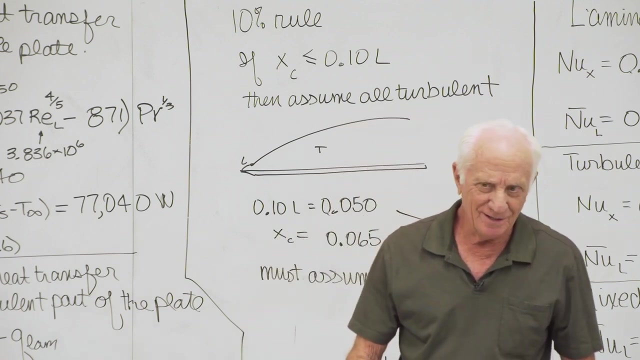 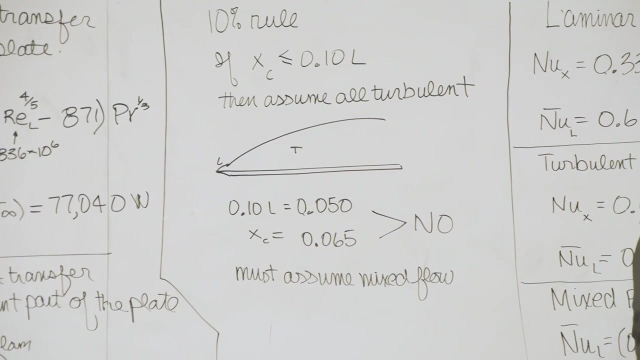 No, Must assume mixed flow over plate. Okay. So the textbook does it similarly, but he uses a five percent rule. I just took 10 percent because it's a little easier to calculate. So what it means is if the laminar part of the plate is really 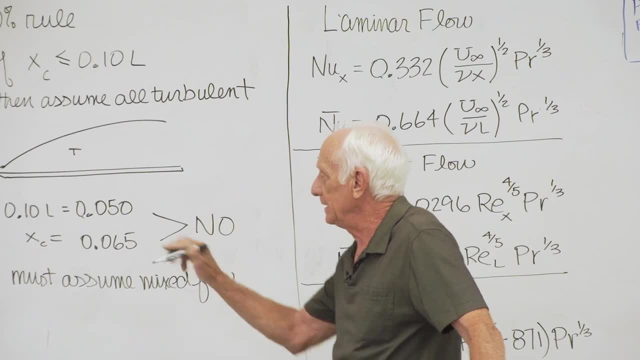 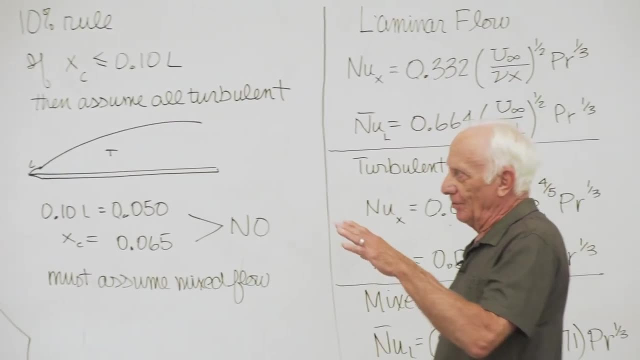 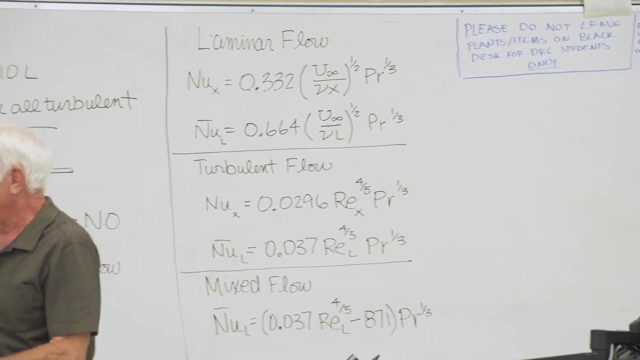 really small compared to the turbulent part. you can neglect that little piece of laminar flow and assume it's turbulent from the leading edge all the way back. Okay, So there are how you use these equations over here for a flat plate flow. Okay, Get the Reynolds number first. 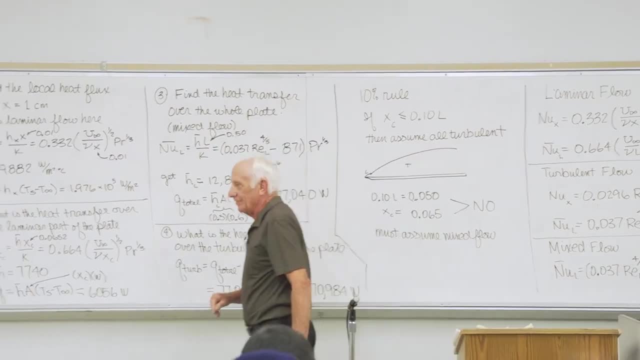 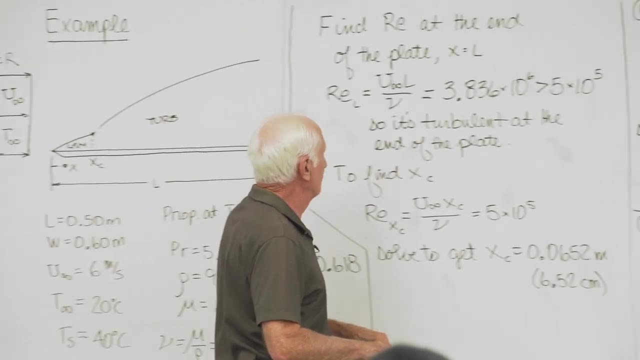 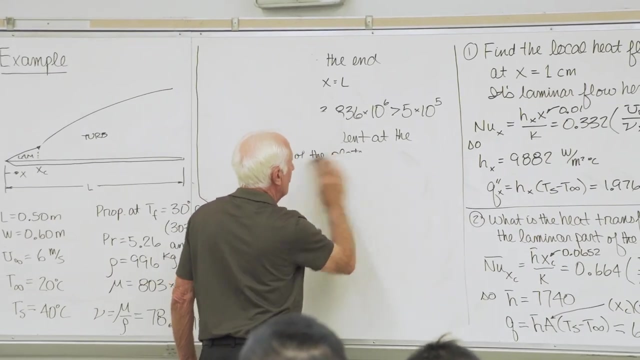 Obviously, that's the key thing. Reynolds, number first. Okay, Any question on that before we go on then? Okay, So we are going to transist to the last part of Chapter 7, external flow- flow over bodies- and we go from a flat plate. 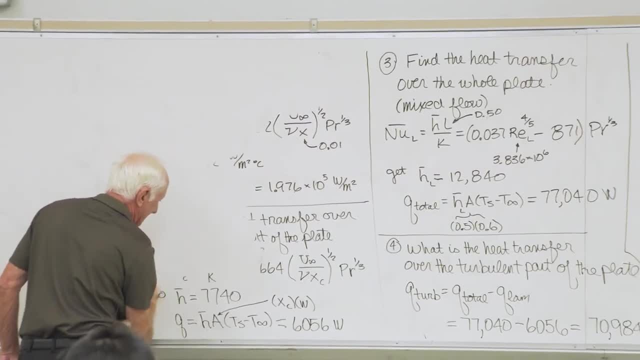 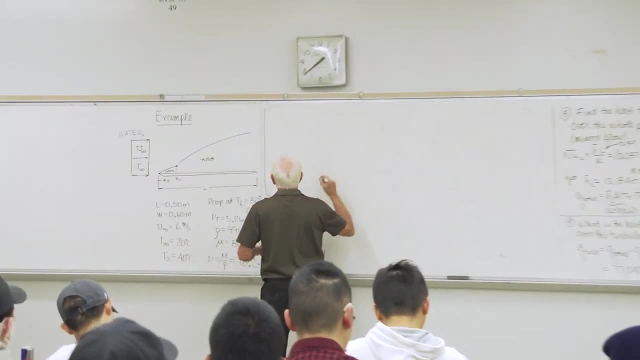 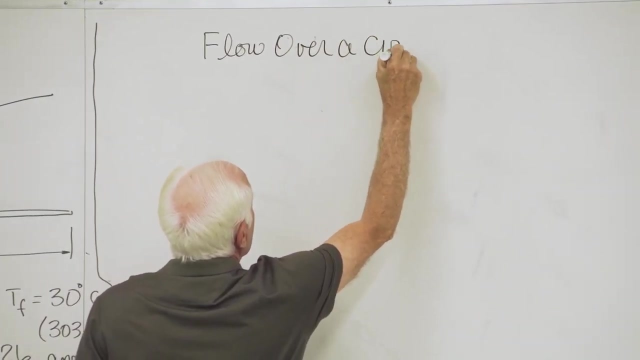 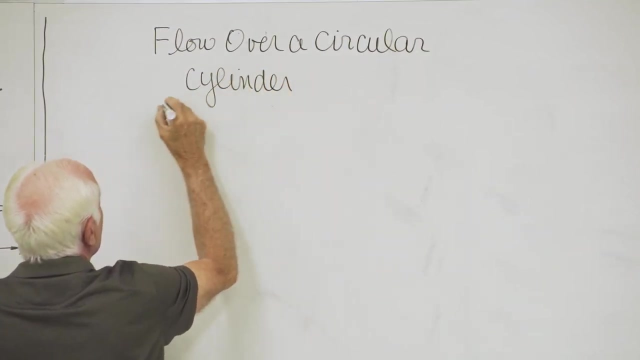 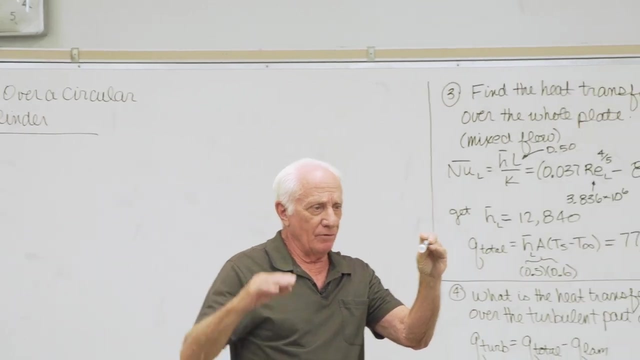 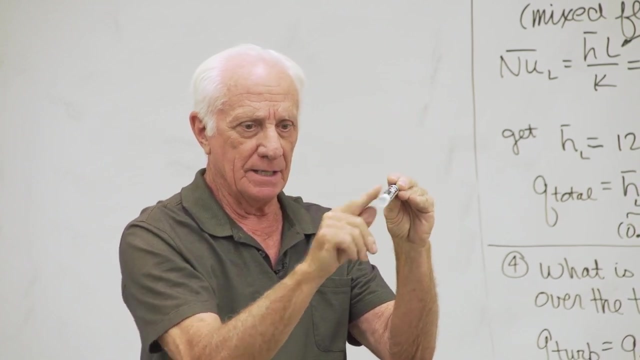 to a circular cylinder. So let's first of all flow over a circular cylinder. So if this pen is a circular cylinder, it is- then we're looking at flow on the outside of the pen. Flow goes over the pen If the pen is hot and the air is cold. 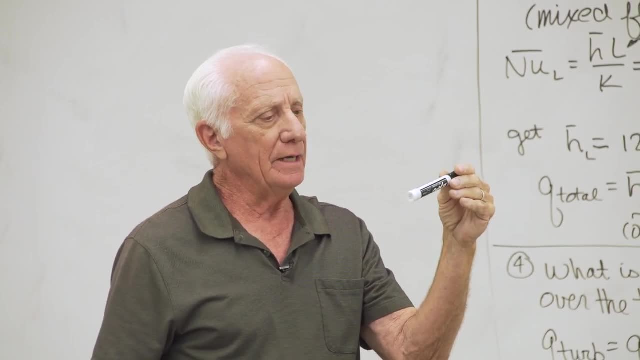 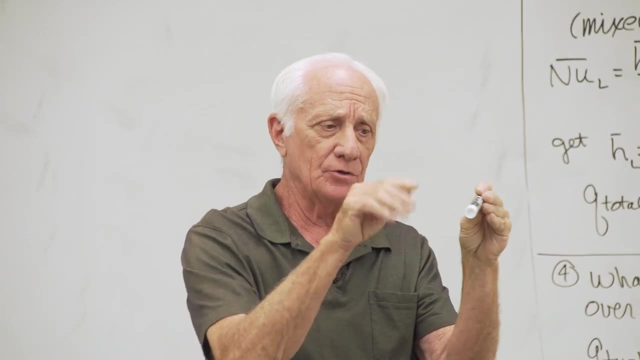 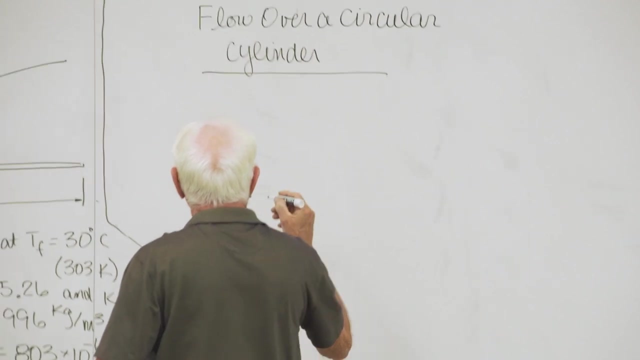 there's heat transfer convection. By the way, Chapter 8 is going to be internal flows, flow of fluids in the tube. Chapter 7 is flow on the outside of the tubes: normal to the tube coming in straight. Okay, So our picture then looks like this: 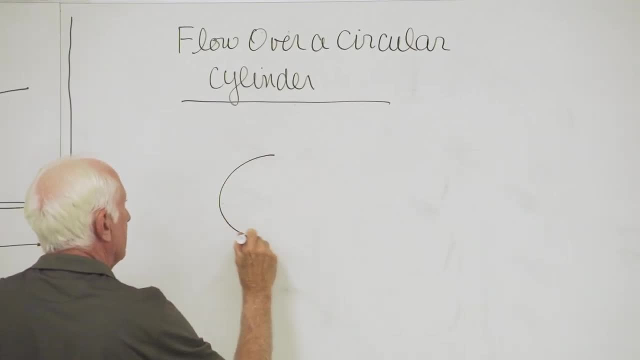 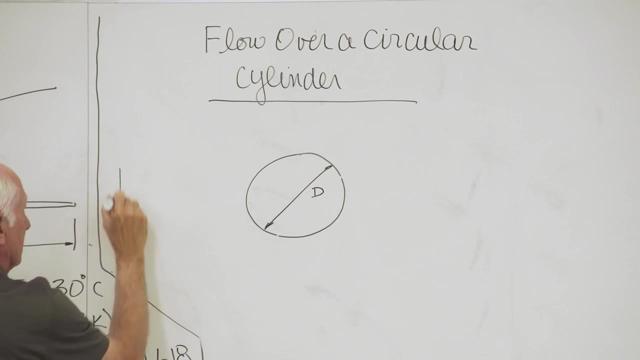 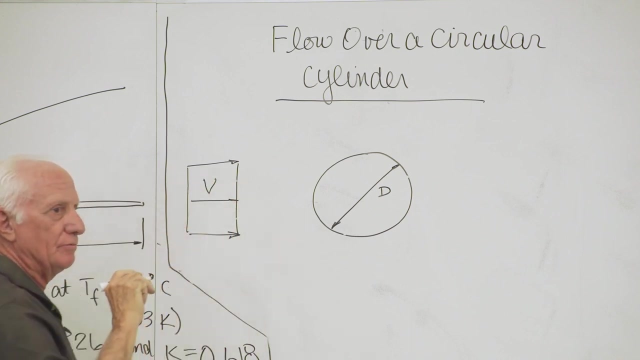 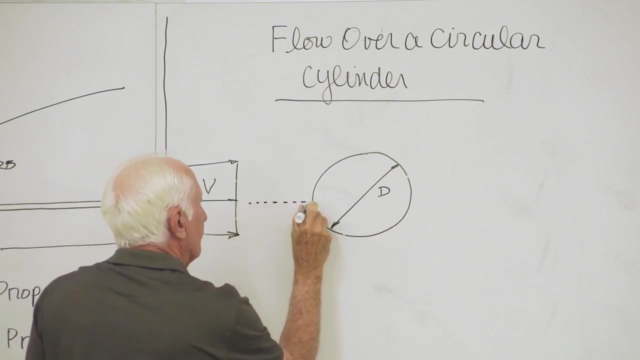 Here's the circular tube. It's diameter is d and the approaching stream looks like this. We don't use u infinity anymore, We use v, the velocity approaching the cylinder. This is fluid mechanics now, because again, you can't do the heat transfer unless you have. 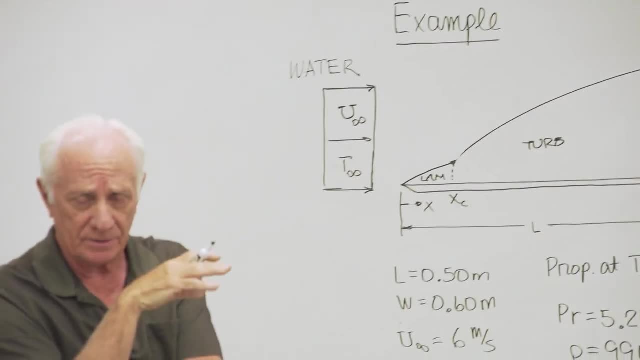 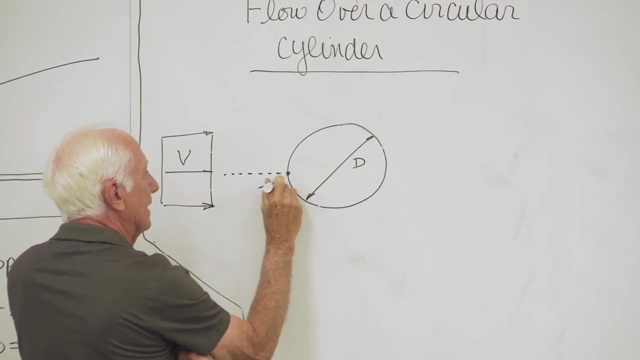 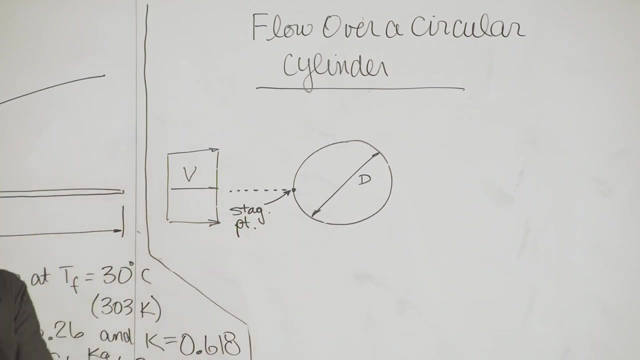 a really good idea of what's going on from the fluid mechanics. That's the fluid mechanics aspect of the problem. When the flow hits this point here, that is the stagnation point. The word stagnate means to be no velocity. Stagnant fluid: it's not moving. 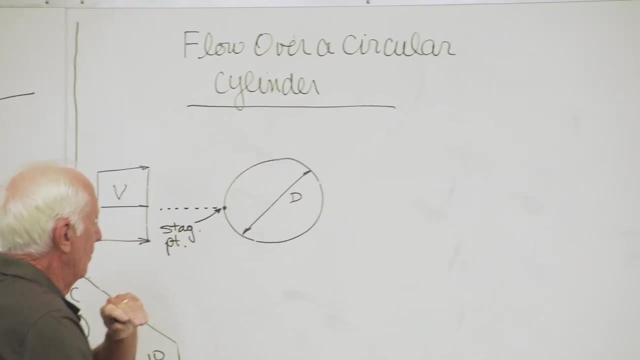 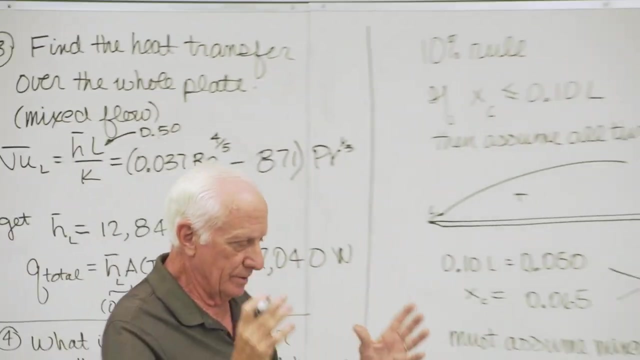 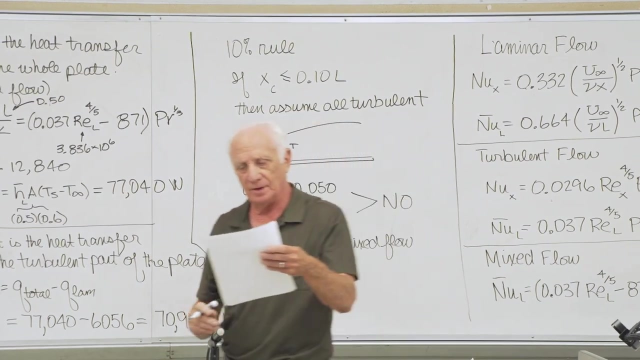 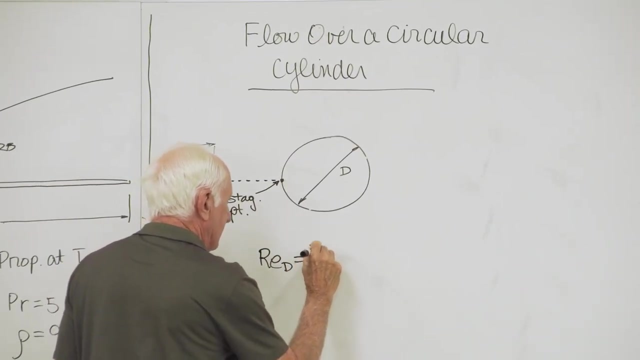 So the velocity is zero there. What happens now is a laminar boundary layer builds up Around the perimeter of the tube. This is for a Reynolds number of about one times 10 to the fourth. So this is for a Reynolds number vd over nu. 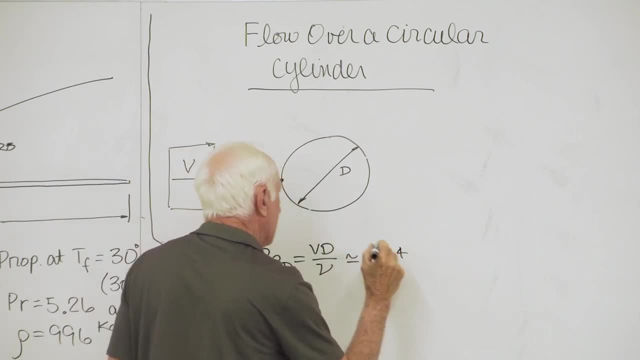 one times 10 to the fourth. So a laminar boundary layer builds up. When it gets to the backside of the cylinder, it breaks off. laminar boundary layer goes around. the cylinder gets to the backside, breaks off. This is a laminar boundary layer. 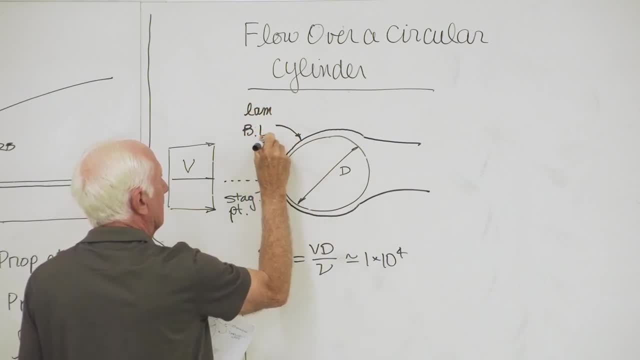 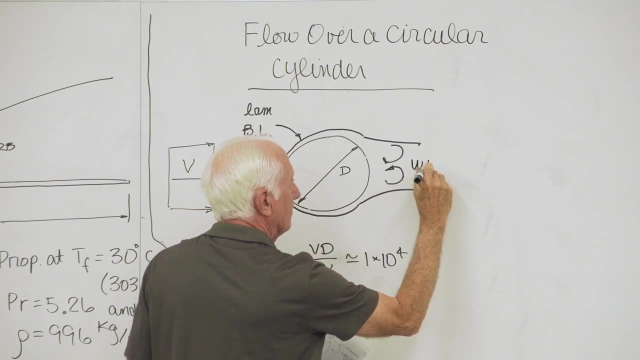 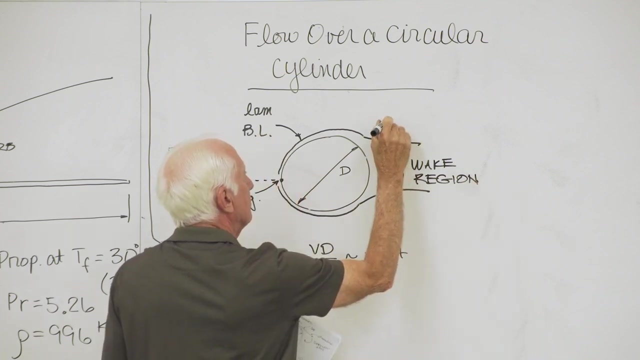 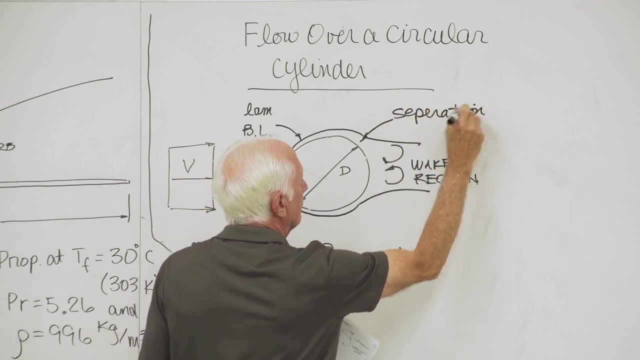 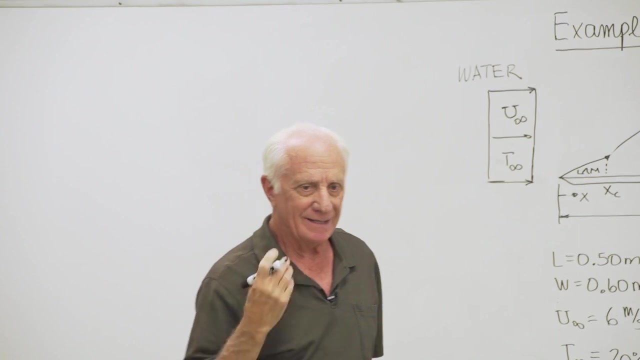 This is what's called a turbulent wake region. This is called the separation point. What does that mean? It's the point where the boundary layer separates from the cylinder. It can't hang on any longer. Its momentum won't overcome the pressure change. 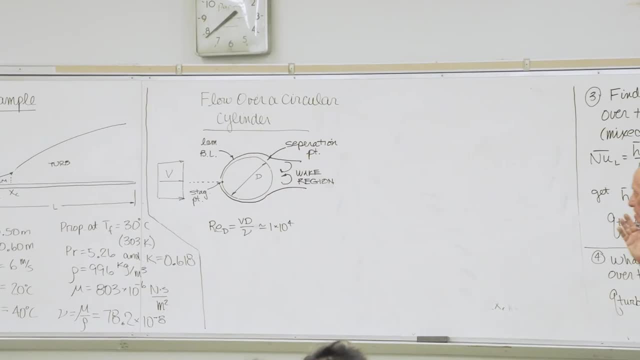 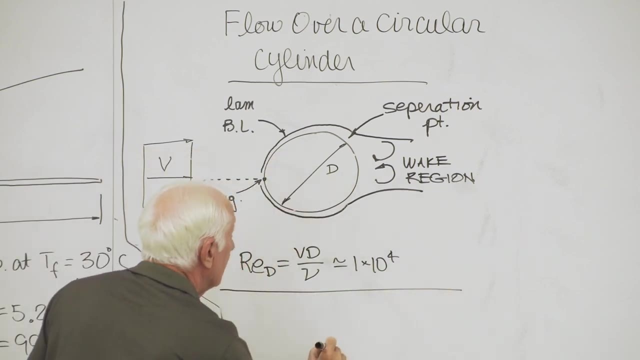 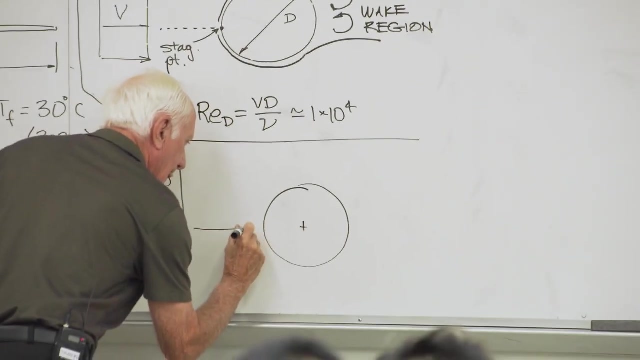 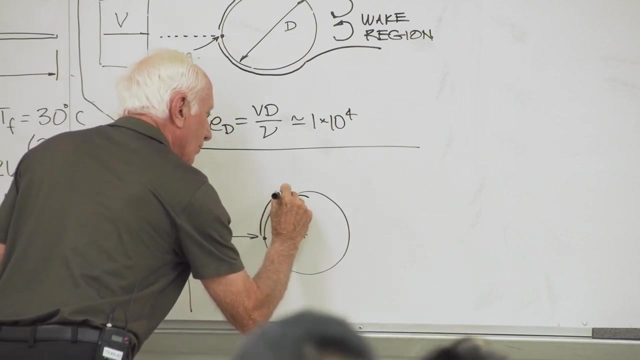 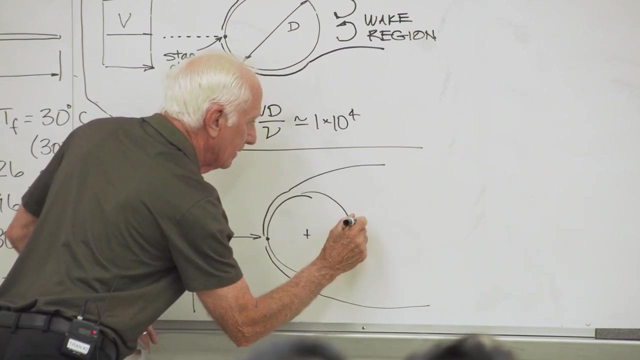 So it just breaks off from the cylinder wall. Then we have another case. Let's draw this one: Spagnation point- laminar boundary layer Separation point- can actually move on the front side of the cylinder. Separation point breaks off like that. 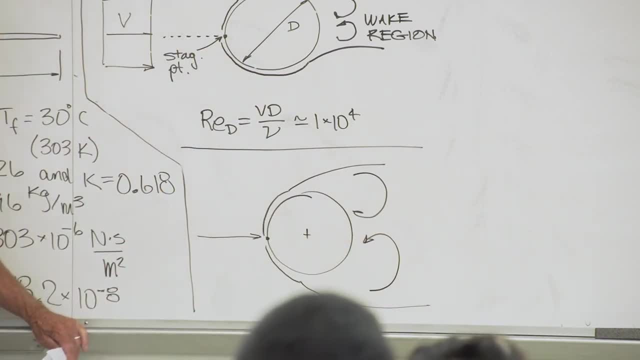 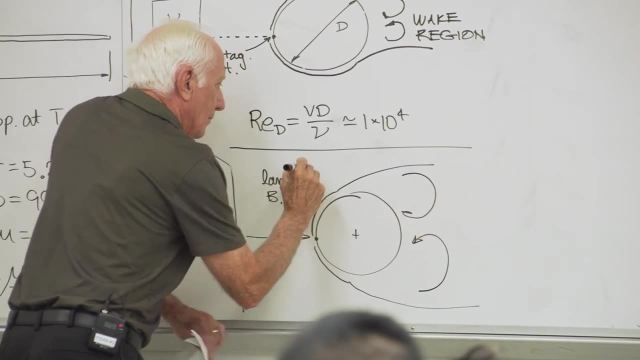 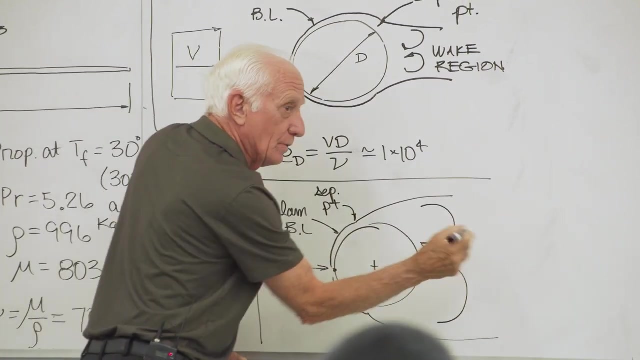 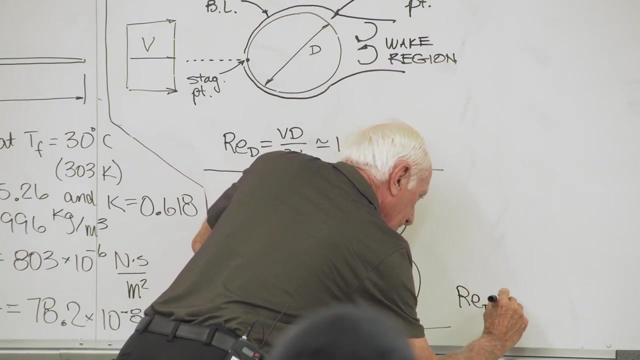 The wake region becomes larger, much larger. the wake region. We still have the laminar boundary layer on the front. We now have the separation point on the front side and then a large wake region behind it. This Reynolds number is about one times 10 to the fifth. 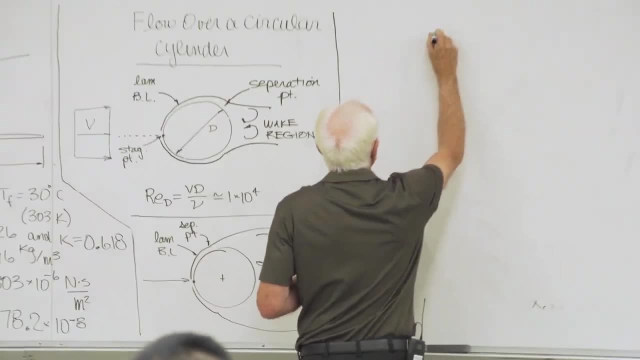 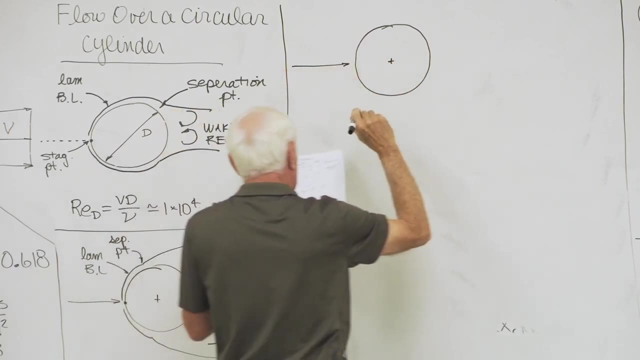 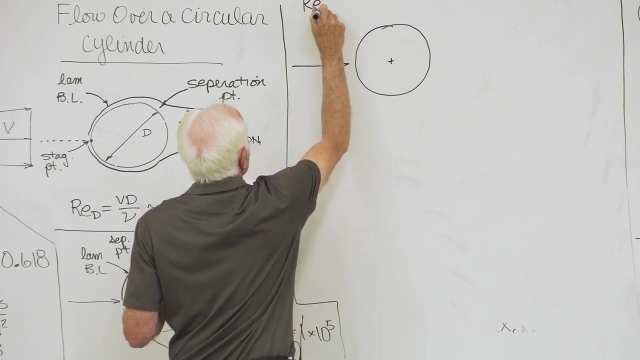 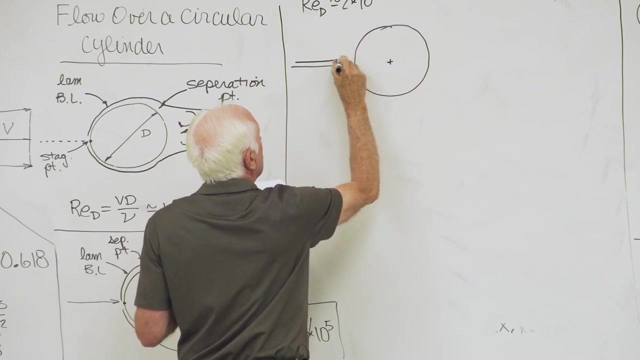 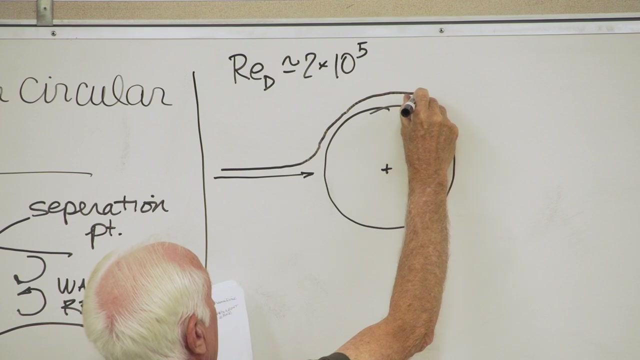 And we'll draw one more Now. this is Reynolds number, about two times 10 to the fifth. At a certain point it transits turbulent boundary layer separation point. 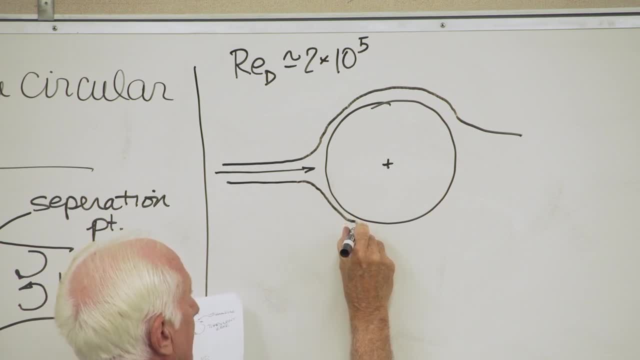 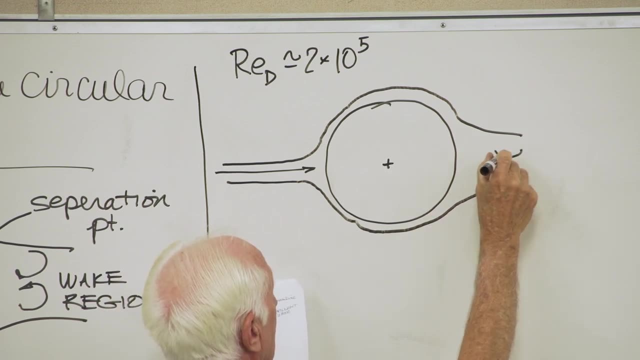 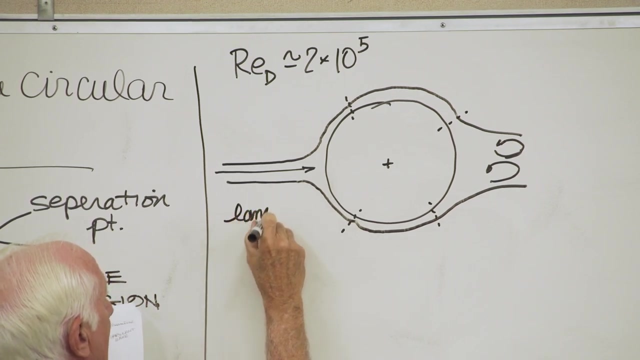 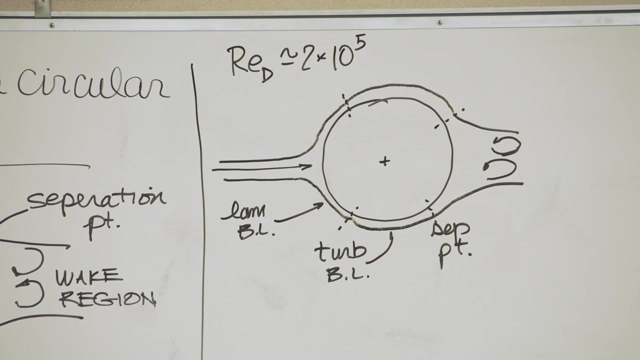 laminar boundary layer. critical Reynolds number for transition to turbulent separation point. Wake region. Laminar boundary layer. turbulent boundary layer separation point. Oh yeah, it's a pretty complicated fluid mechanics situation. Is there a magic Reynolds? Well, flat plate flow. 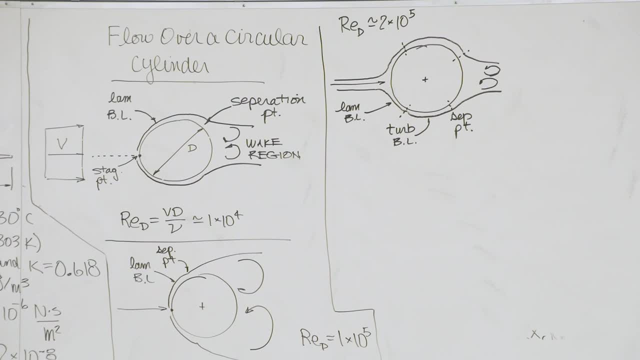 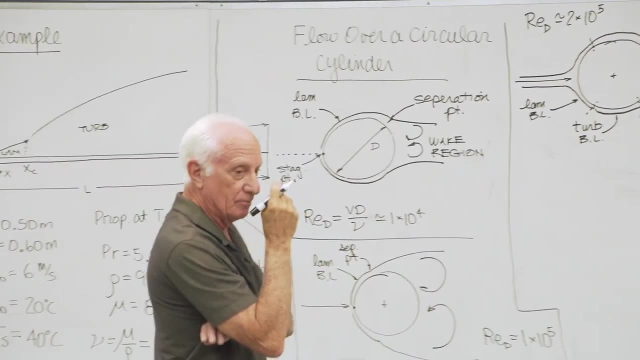 Is there a magic Reynolds? No, The flow changes to pay on the Reynolds number. Yeah, 500,000.. X critical. Is there a magic Reynolds number for flow over a cylinder? No, The flow changes to pay on the Reynolds number. 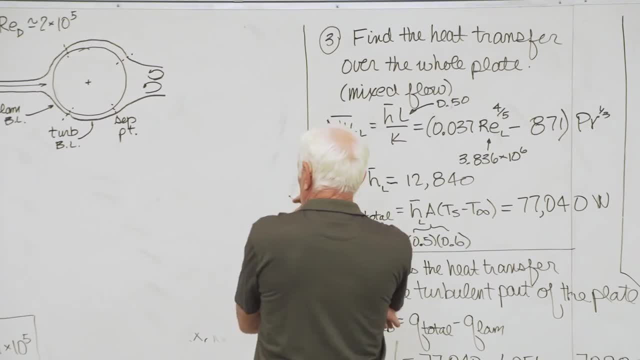 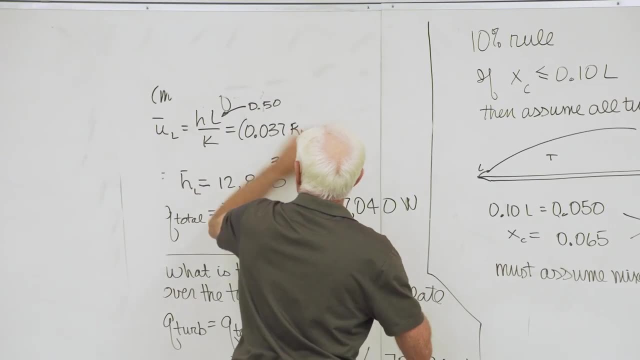 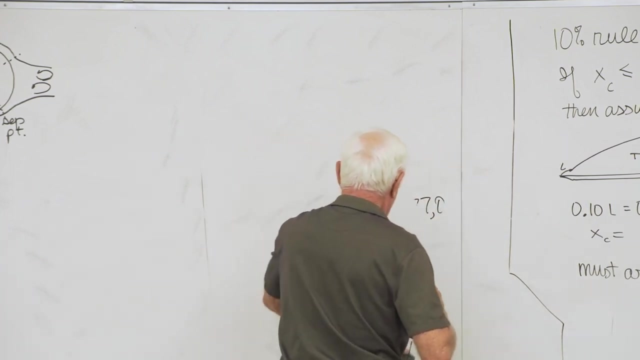 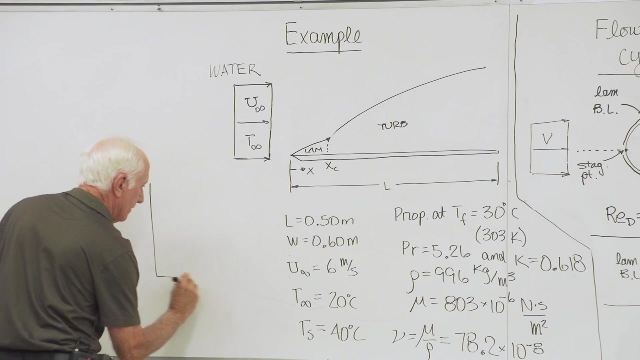 There's no one magic Reynolds number. Okay, so now you know, life becomes more complex, obviously. How does the convection coefficient vary? Oh, you know, for a flat plate we knew how H varied HX versus X. 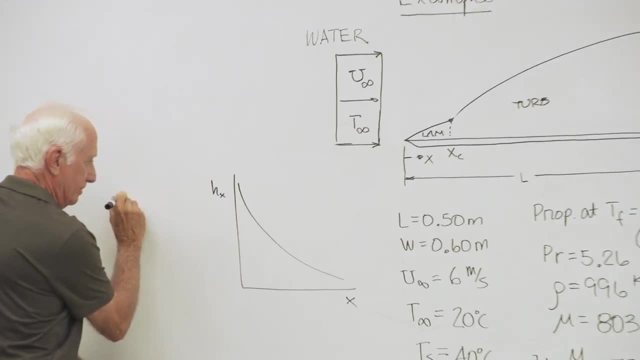 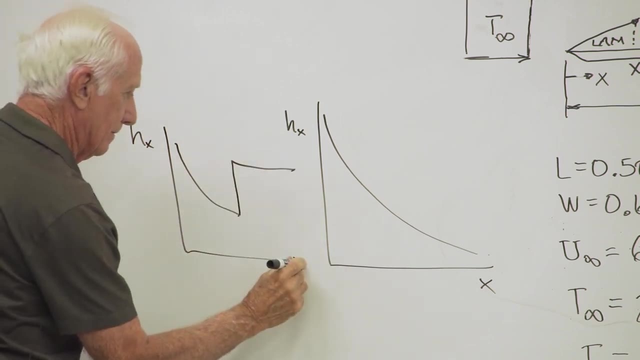 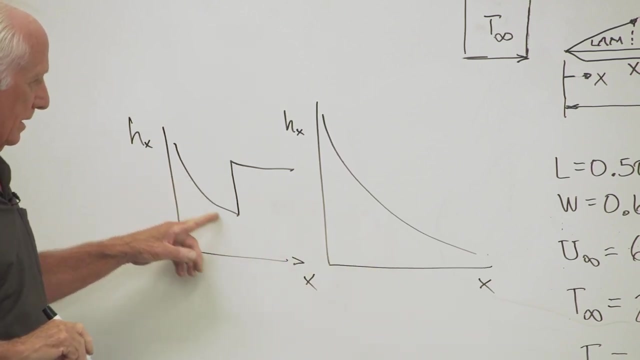 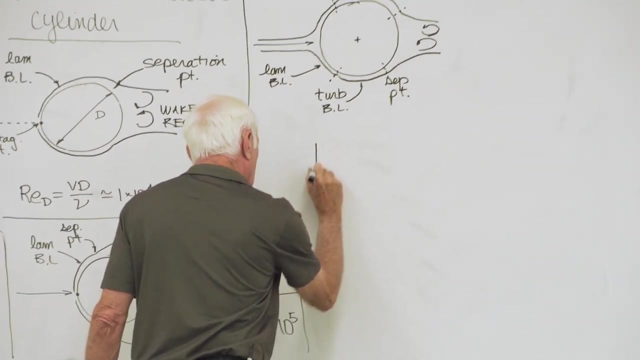 Or maybe it looked like this turbulent flow flat. That's how laminar flow, mix flow, laminar transist, turbulent. Okay, how does this look when we plot H here? We don't call it HX. 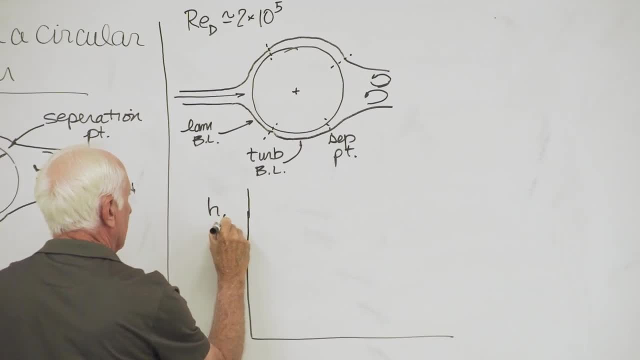 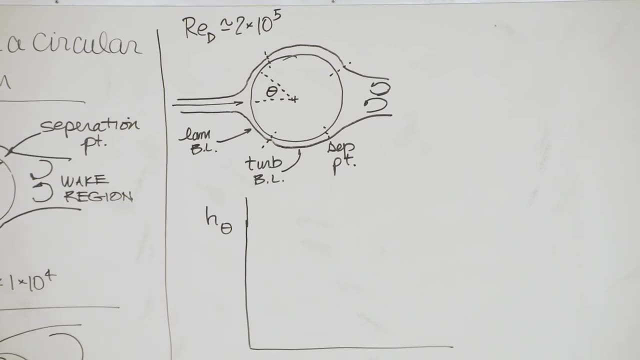 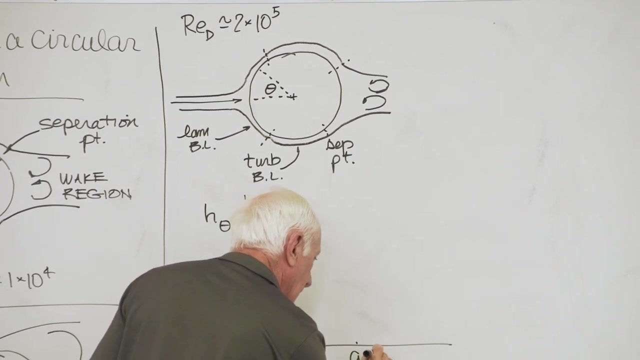 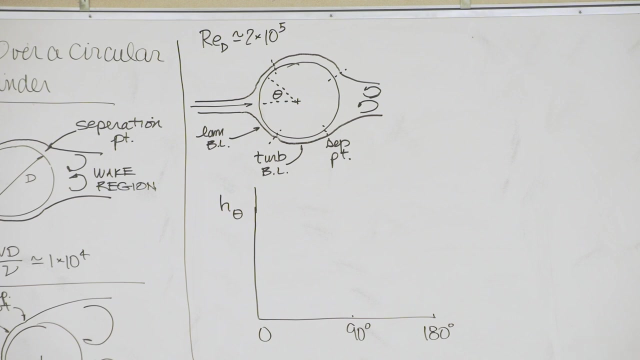 We call it H theta. Where theta is measured from the front stagnation point, Theta equals zero. So 0, 90 degrees 180.. Let's pick a particular Reynolds number. Here we go First. one we'll take is Reynolds of 1 times 10 to the 4th. 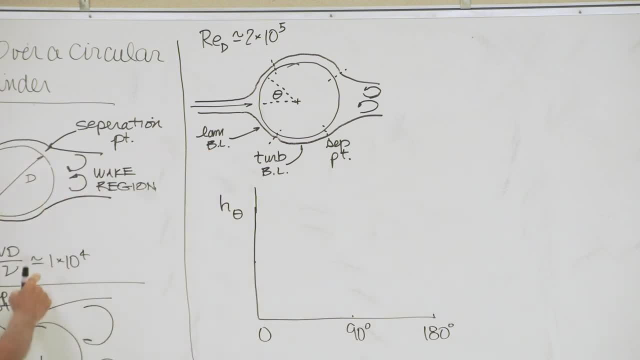 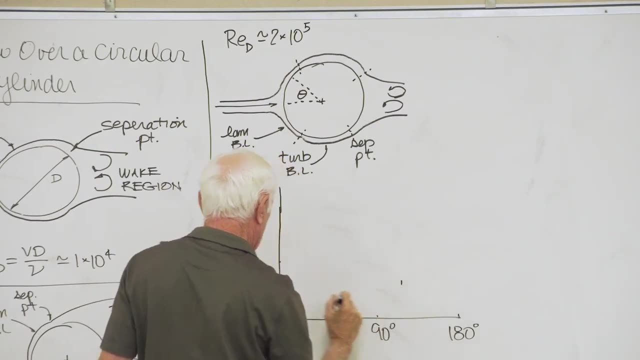 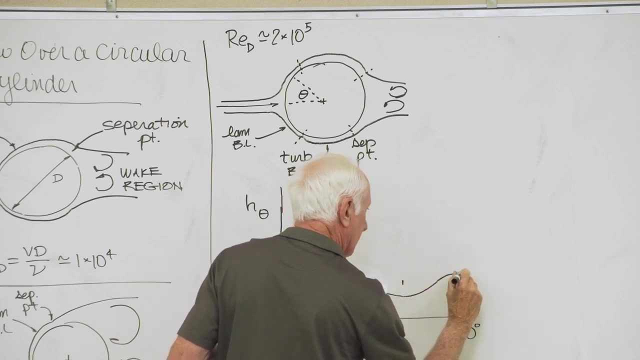 So it looks something like this: 1 times 10 to the 4th. that's here Separation point occurs on the back side, on the back side past 90, back here somewhere. So it goes down, it hits the separation point and it goes back up again. 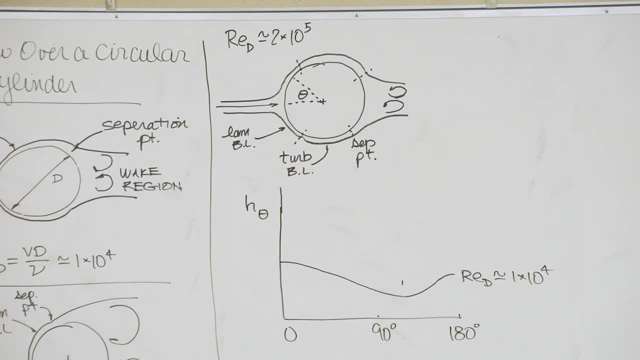 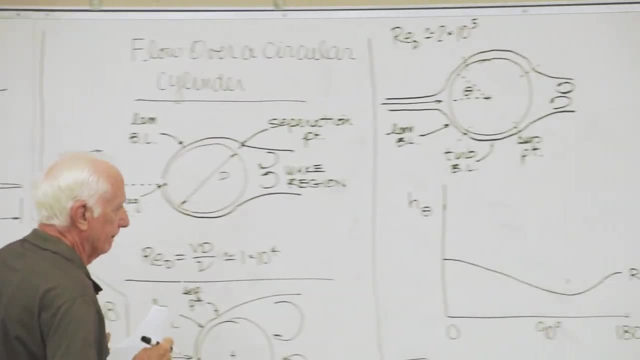 Okay, The wake region creates a bigger H value because it's a very turbulent region. Turbulent eddies are in that region, They're swirling. Let's go to Reynolds, number 2 times 10 to the 5th- This guy up here- 2 times 10 to the 5th. 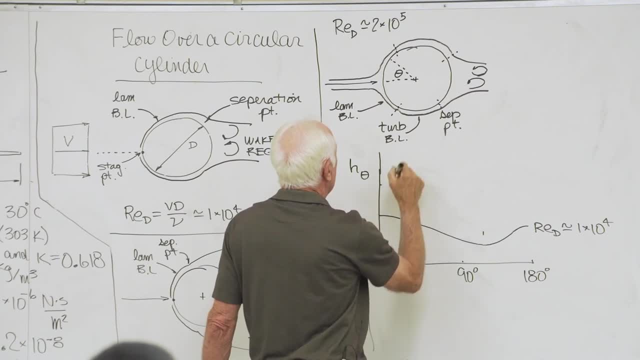 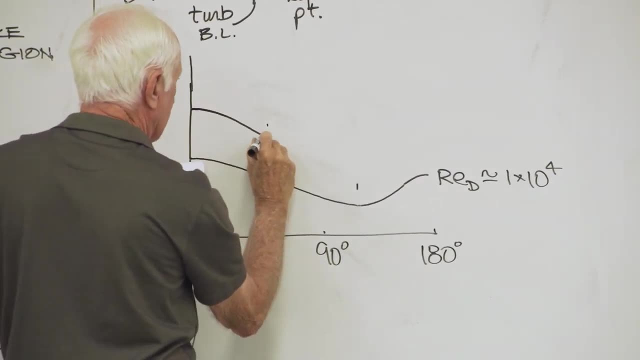 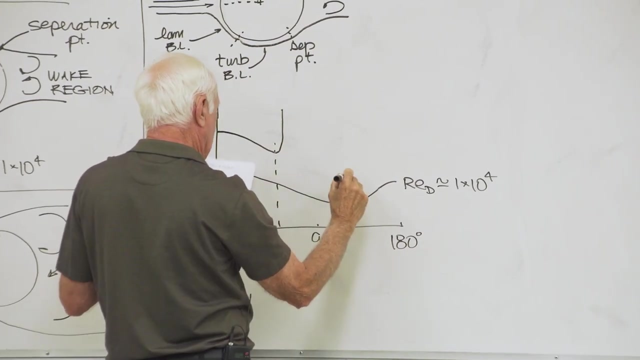 Oh yeah, H gets bigger now because the Reynolds number is bigger. Now we go through a turbulent location where the flow transists to turbulence. It goes up. It goes up because now turbulent gives greater heat transfer coefficient. Then it goes back down again to separation point, and separation point occurs way back here. 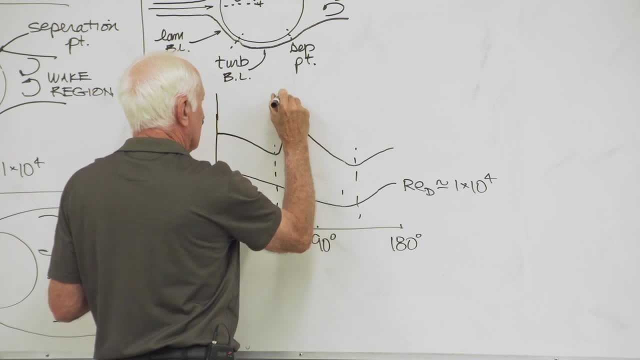 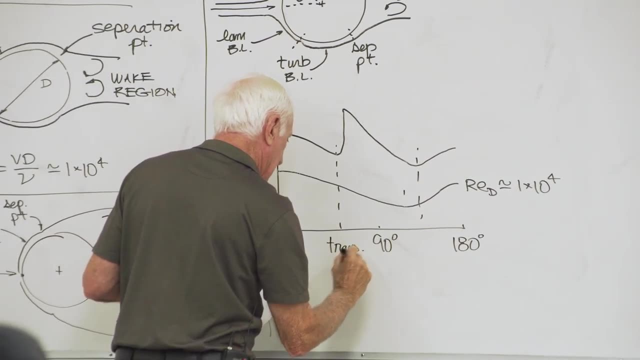 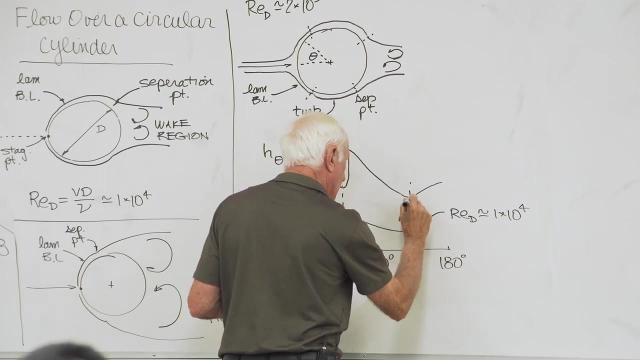 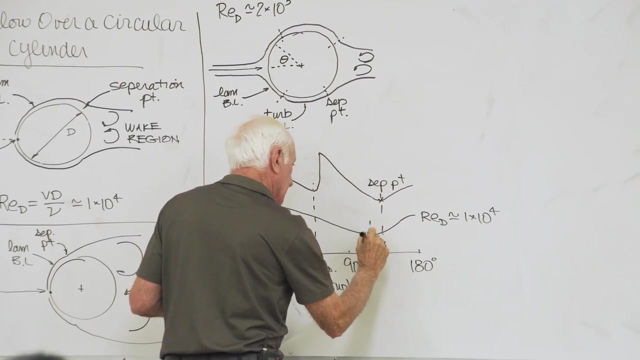 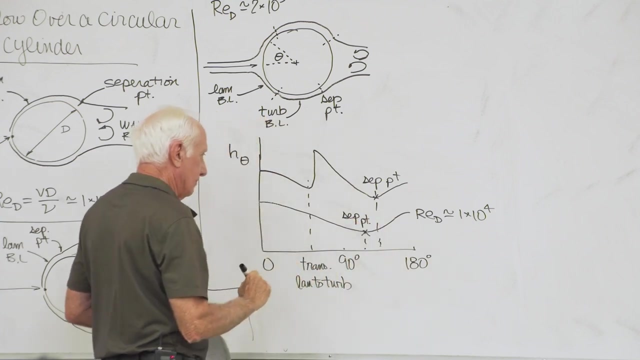 It hits here, Then it goes back up again. So this is transition: Laminar of turbulent. This is the separation point for this guy. This is a separation point for this guy And you can see when the boundary layer transists from laminar of turbulent. 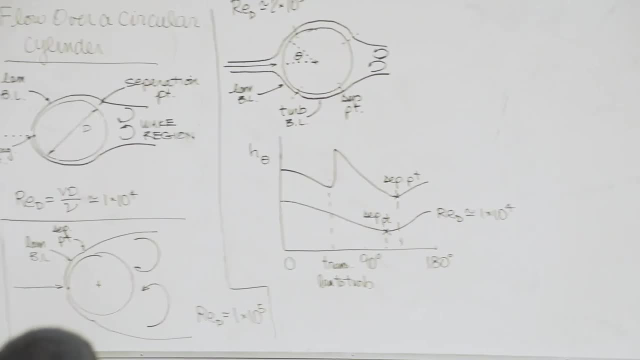 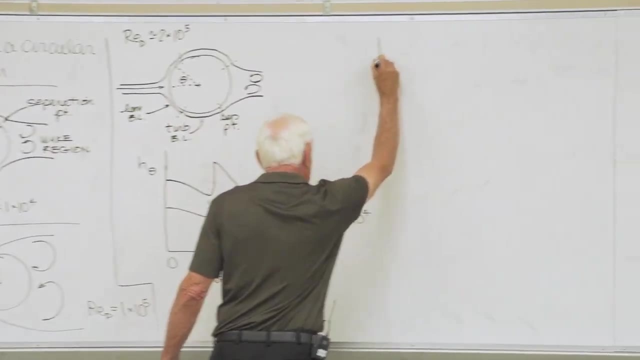 oh bang, it goes up really big. H goes up really big. So that's what happens in the heat transfer And the heat transfer part of the problem. as you can see, Just like a flat plate with the two figures over there, how does H vary with X?